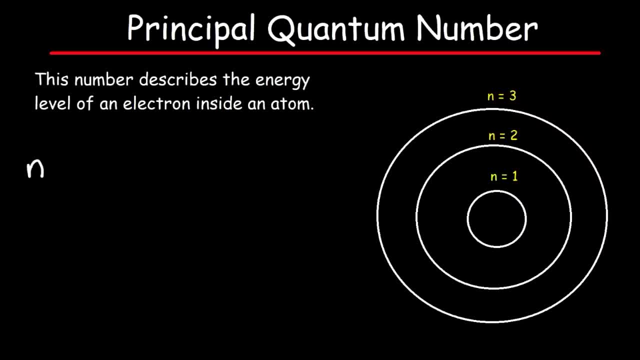 The first one is n. n is the principal quantum number And n is an integer- 1,, 2,, 3,, 4, and so forth. n can be zero. The principal quantum number describes the energy level of an electron inside an atom. So, looking at the picture on the right, we basically have: 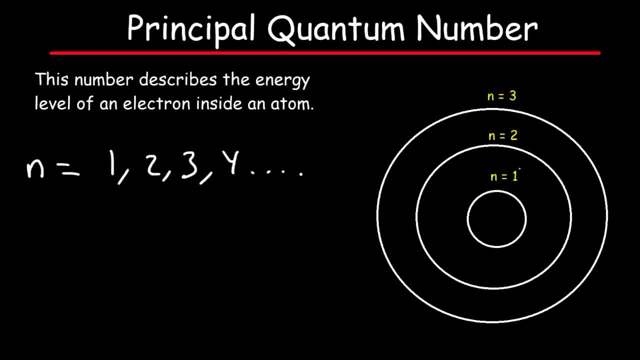 a Bohr's model of the atom, And we can see that the first shell represents the first energy level, The second circle is the second energy level where n is 2.. And the third circle is the third energy level where n is 3.. And so that's the first number you need to be familiar with. 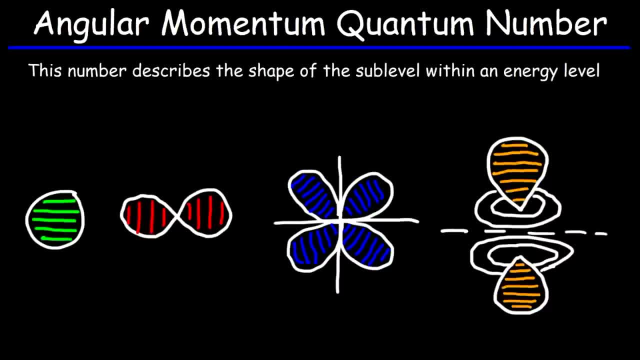 the principal. Now, the next quantum number that you need to be familiar with is the angular momentum quantum number. This number is indicated by the symbol L And it describes the shape of the sublevel within an energy level. Now we have four different sublevels that you're. 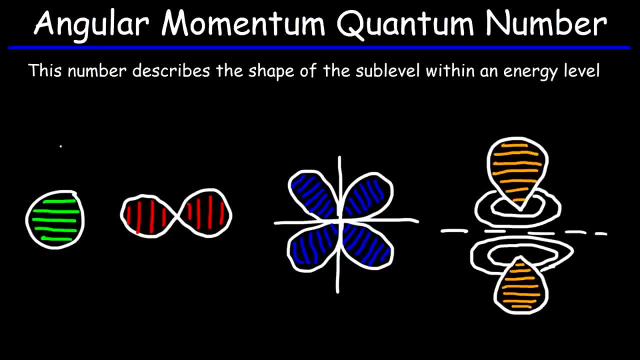 going to see on a regular basis. The first one is the s sublevel, which is basically a sphere. The second one is the p sublevel, And then we have the d sublevel and the f sublevel. Now, what you need to know is that for the s sublevel, L is always zero. For p, L is. 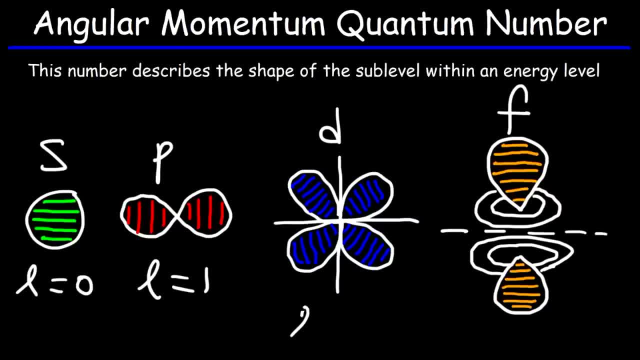 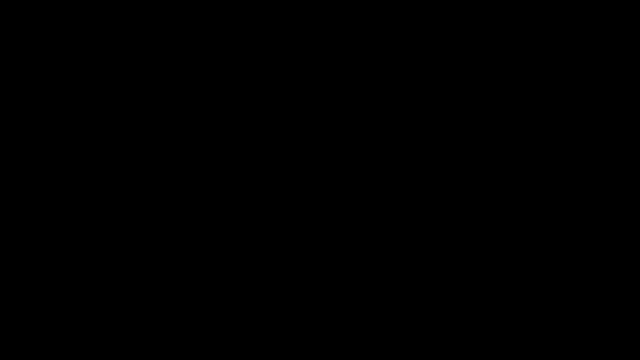 1.. For d the angular momentum quantum number is 2. And for f L is always 3.. Now let's talk about the relationship between n and L. L is less than or equal to 1.. L is less than or equal to n-1.. And L and n are both integers. So let's talk about what. 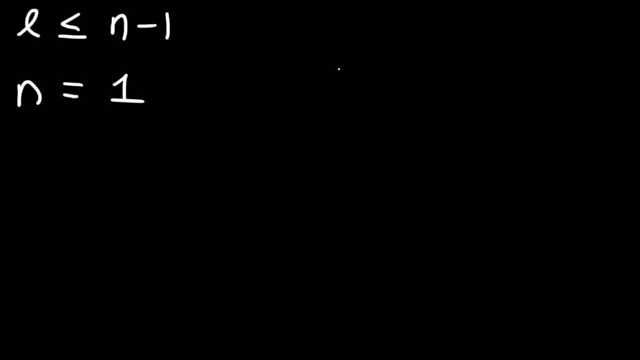 this means When n is 1, L can only have one value, That's, n-1 or 1-1,, which is 0. Now, when n is 2,, according to this equation, here L has to be less than or equal to n-1. 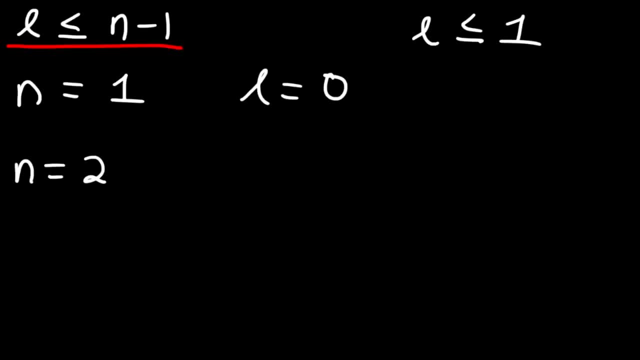 or 2-1, which is 1.. So that means L could be 0.. L could be 0 or 1.. And this expression will be true. Now, what about when n is 3?? When n is 3, the maximum that L can be is 3-1 or 2.. 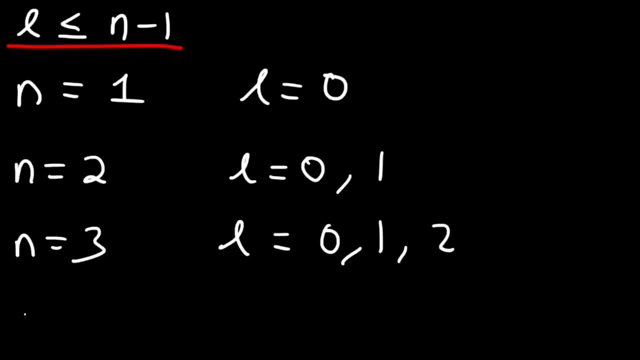 So L can be 0,, 1, or 2.. When n is 4,, L could be 0,, 1,, 2, or 3.. Now let's think about what this means. So remember, When L is 0,, what sub-level do we have? 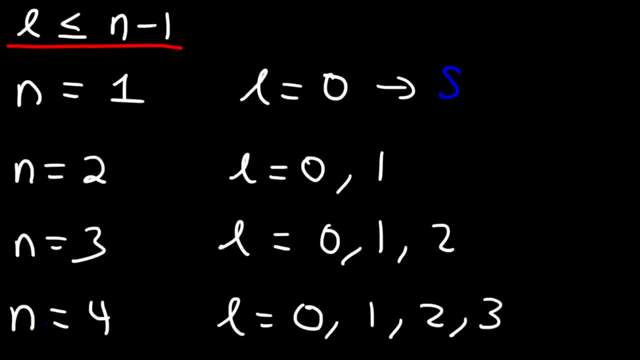 When L is 0, this corresponds to S. Now, when n is 2, L could be 0 or 1, which means that we could have the S or the P sub-level. When n is 3,, L could be 2, so we could have the S, P or D sub-level. 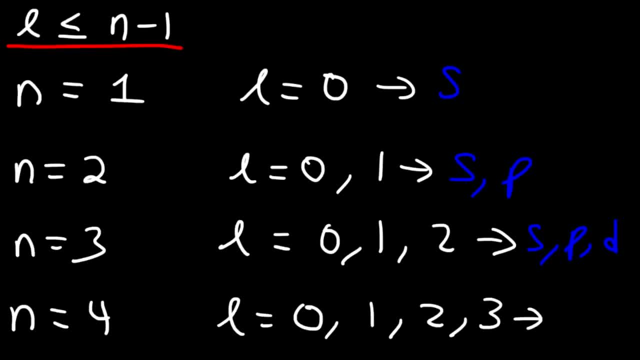 When n is 4, we can have the S, PDP or D, performance or F sublevels. Now notice that there's no 1P sublevel. This does not exist. The first energy level doesn't have the P sublevel. And let's say, if you were to write the electron configuration, 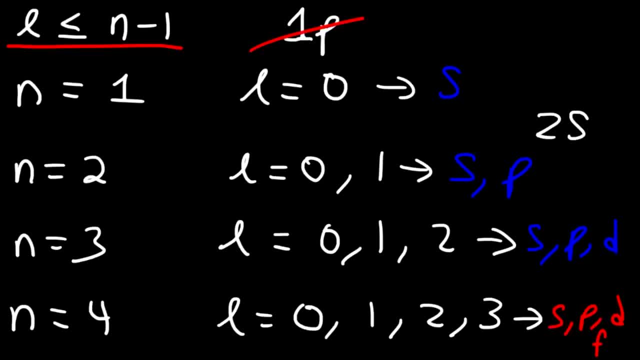 for an element. you'll know that there is no 2D sublevel. You have 2S and 2P, but not 2D. In the third level you could have 3S, 3P, 3D but not 3F. So 3F is not possible Now you could. 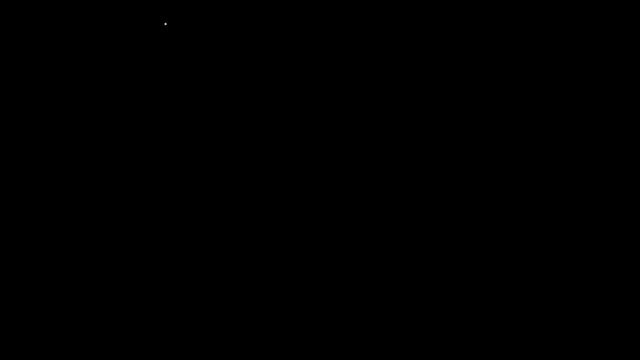 have 4F. That's possible. Now here's a question for you. Let's say we have an electron in the 3D sublevel. Based on that information, what is the N value and the L value that corresponds to an electron in the 3D sublevel? 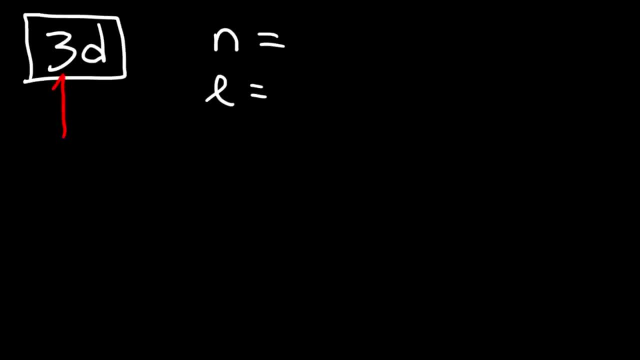 N is basically the number that you see here. So N is 3.. Now for the D sublevel: L is what value? So, if you recall, for the S sublevel, L is always 0.. For the P sublevel, L is 1.. For the D sublevel: 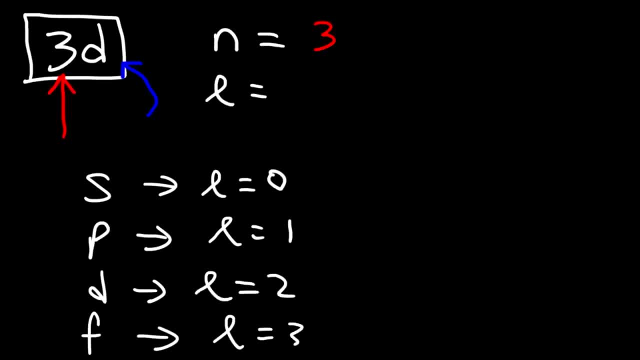 L is 2.. And for the F sublevel, L is always 3.. So for the 3D sublevel, N is 3 and L is going to be 2.. So let me give you another example. What if we have an electron in the 4F sublevel? What's N and 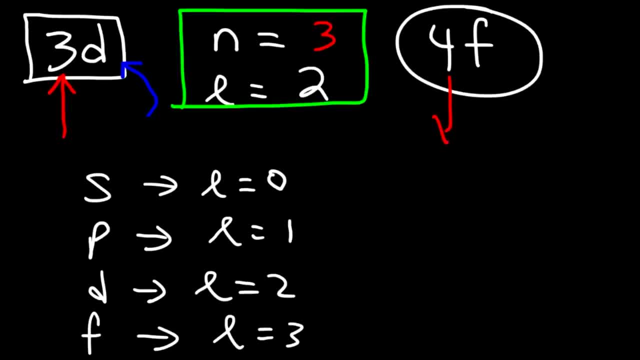 what's L? As we can see, N is the number in front of F, So N is 4.. And F always corresponds to an L value of 3.. So for an electron in the 4F sublevel, N is 4, L is 3.. Now let's move on to the third. 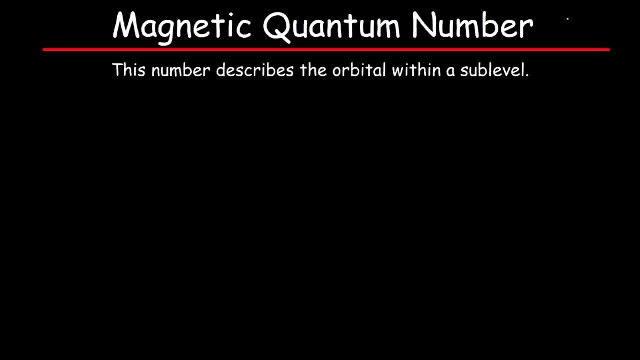 question. So let's talk about quantum number, which is the magnetic quantum number represented by the symbol M sub L. This number describes the orbital within a sublevel. An orbital is basically a region in space in which the probability of finding an electron is very high. In an orbital, an electron 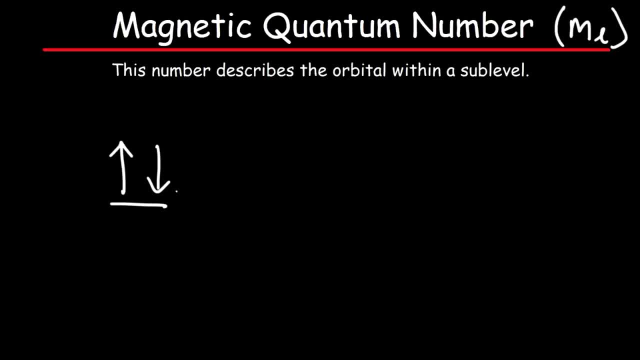 can have an upspin or a downspin, And so every orbital can hold a maximum of two electrons. But now let's talk about quantum number. So let's talk about the relationship between L and M sub L. So, as we said before, L is the angular. 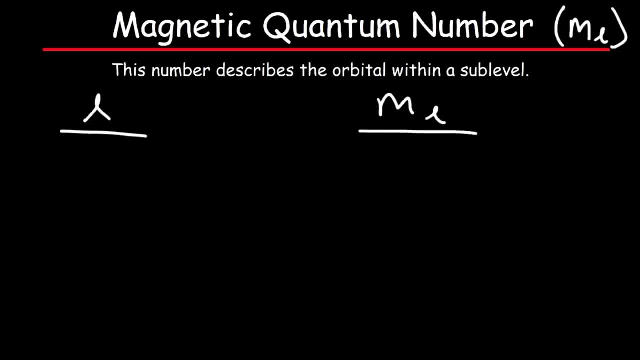 momentum quantum number. M sub L is the magnetic quantum number. So when L is 0,, we have the S sublevel And ML can only be 0.. When L is 1,, we have the P sublevel And the P sublevel has three. 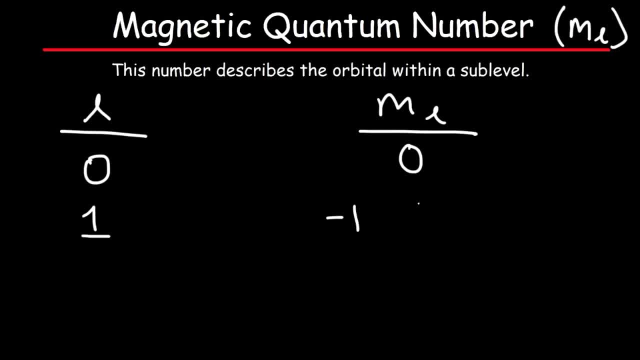 orbitals. The first one has the ML value negative 1.. The second one is 0.. And the second one has the 0.. And the third one has an ML value of 1.. When L is 2,, we have the D sublevel, And there are five. 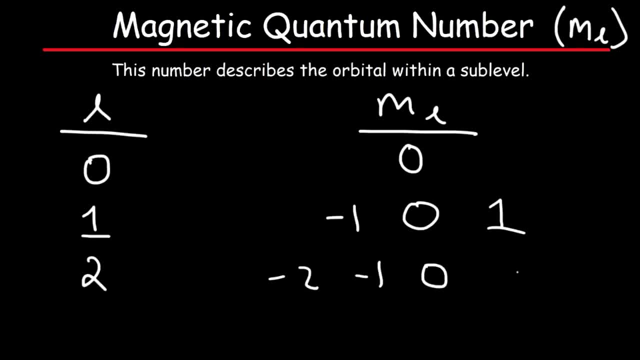 D orbitals negative 2, negative 1,, 0,, 1, and 2.. When L is 3,, we have the F sublevel, which has seven orbitals: negative 3, negative 2, negative 1,, 0,, 1,, 2, and 3.. So what you need to know is this: 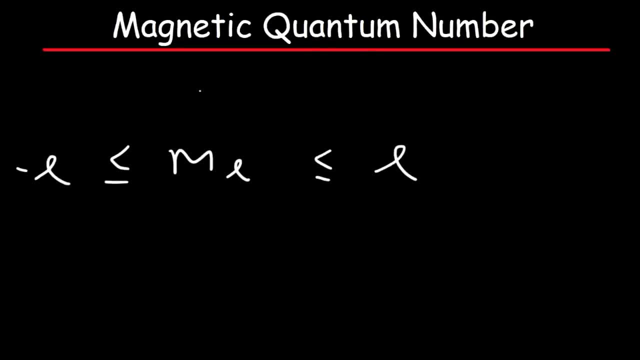 Between negative L and L. So let's say, if L is 4, that means ML will be an integer between negative 4 and 4.. So it could be negative 4, negative 3, negative 2, negative 1,, 0,, 1, 2, 3, 4.. So this 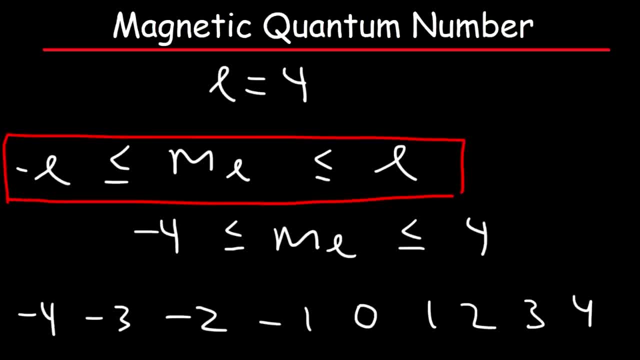 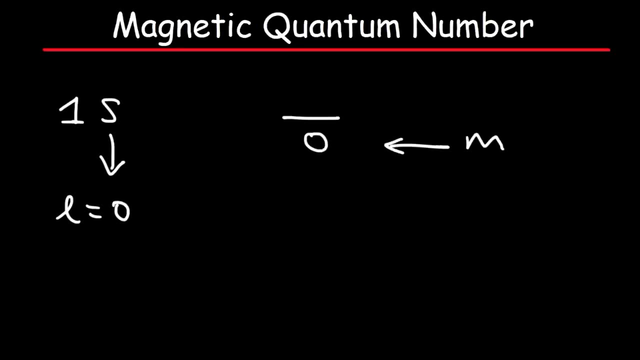 expression shows the relationship between ML and L. So let's say, if we have the 1S sublevel, S only has one orbital And for S, L is 0.. And ML, which is this number, will also be 0.. 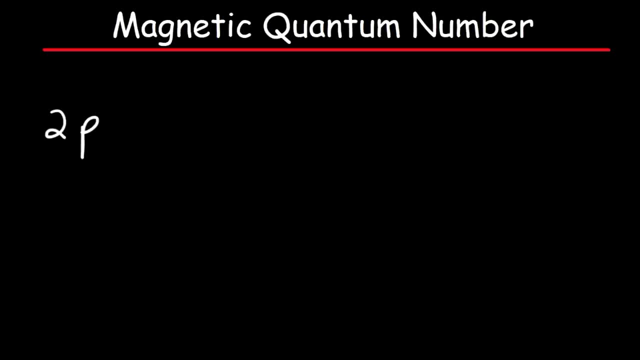 Now let's say, if we're focused on the 2P sublevel, P has three orbitals. Now, for 2P, we know that N is 2. And for P, L is always 1.. Because L is 1, ML could be negative: 1,, 0, or 1.. And so, as you can, 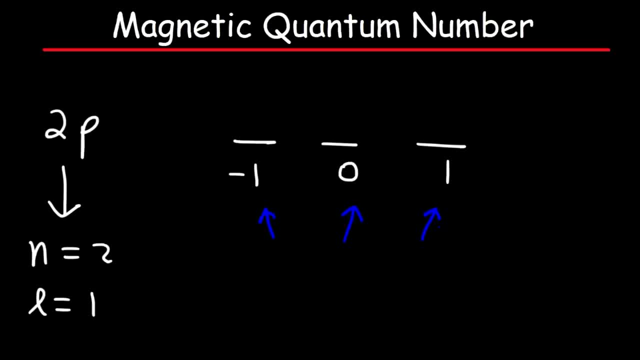 see the ML values. they correspond to the specific orbitals within a sublevel. Now let's say if we have the 3D sublevel where N is 3 and L is 2. Now the D sublevel has five orbitals, which means: 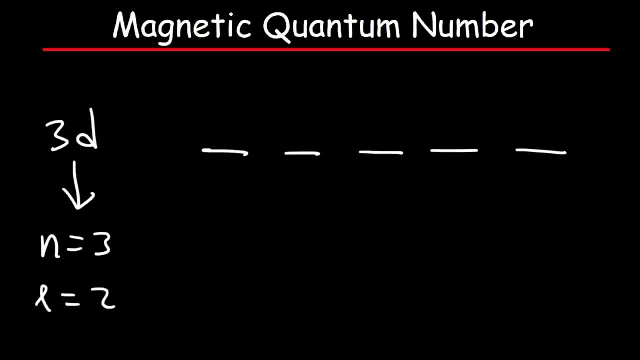 that it can hold a maximum of 10 electrons, because you can put two electrons per orbital. Since L is 2, ML could be anywhere from negative 2 to 2.. And so each ML value corresponds to a specific orbital in the sublevel. Lastly, let's go over 4F, where N is 4 and L is 3.. 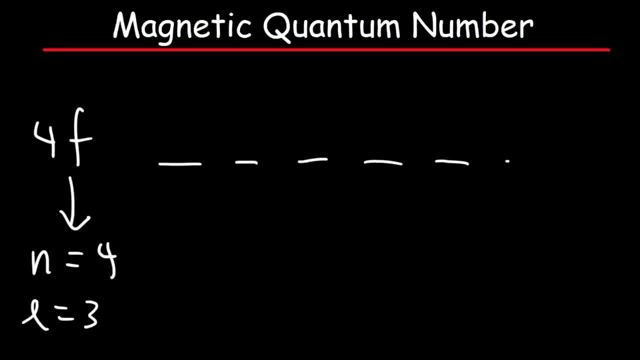 The F sublevel has seven orbitals where ML can vary between negative 3 and positive 3.. So hopefully this helps you. This helps you to see the relationship between L and ML, which gives you these numbers. Now, the last quantum number that we need to talk about is something known as the electron spin. 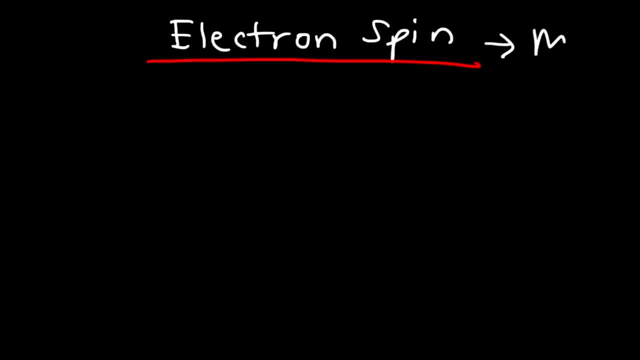 The symbol that corresponds to this is M sub S. Now the electron spin could be one of two values: positive or negative, one half. Now recall that an electron within an orbital can either be going up or down. So if it's going up, the spin is positive one half, And if the arrow, 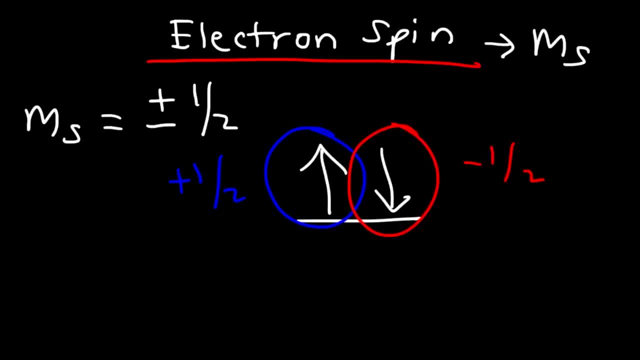 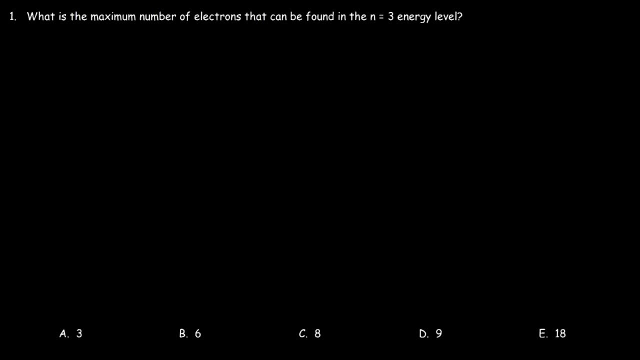 is going down. the electron spin is negative one half, So that's the last quantum number that you need to be familiar with. So here's one problem: What is the maximum number of electrons that can be found in the N equals 3 energy level? Now, for each of these questions you can pause the video. 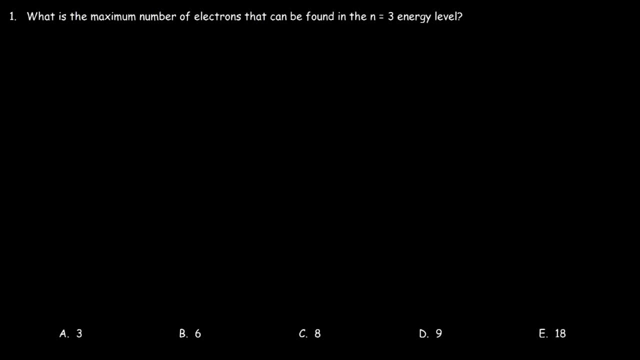 and try it yourself first, And then unpause it to see the solution. So how can we find the answer? The quick and simple way is to use an equation. The maximum number of electrons in a certain energy level is equal to 2 N squared. So 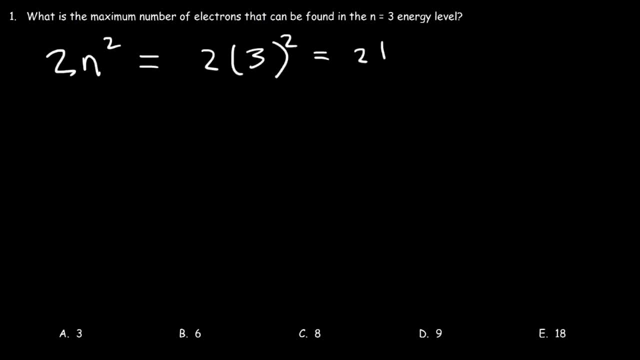 it's going to be 2 times 3 squared, which is 2 times 9.. So that's 18.. So, therefore, E is the right answer. Now, if you want to understand it, you need to know that in the first energy level, 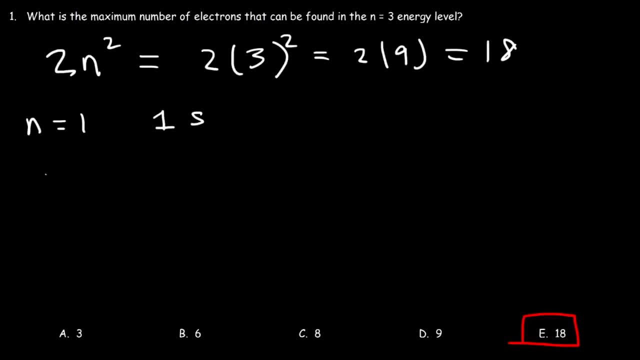 you have only one sublevel, the S sublevel. In the second energy level you have two sublevels: S and P. In the third energy level there are three sublevels: S, P and D. Now S holds two electrons. 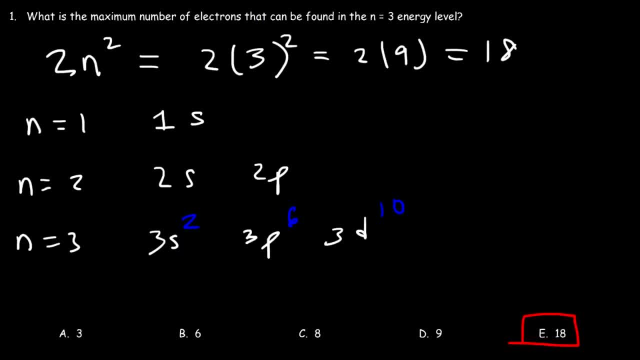 P holds 6,, D holds 10.. So if you add up these numbers- 2 plus 6 plus 10, that's going to give you 18.. This one, Which of the following sublevels, corresponds to the quantum numbers? N equals 3 and L equals 2?? 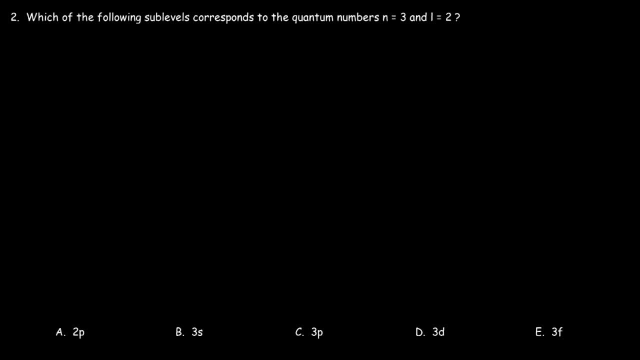 Is it 2P, 3S, 3P, 3D or 3F? You need to know that when L is 0,, it corresponds to the S sublevel. When L is 1,, it corresponds to. 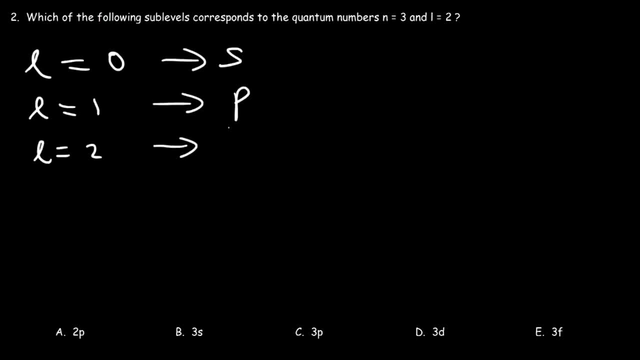 the P sublevel. When L is 2,, it corresponds to the D sublevel, And when L is 3, it's for F. So N is 3, so we have the first number 3.. And when L is 2, we're dealing with the D sublevel. 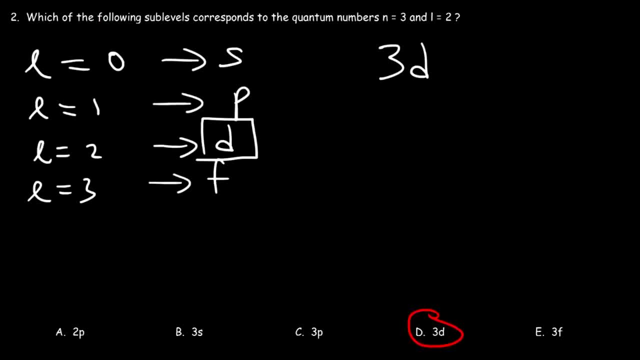 So this is going to be 3D. Now let me give you some more examples on this. So let's say, if N is 4 and L is 3. Go ahead and write the designation or the sublevel that it corresponds to. 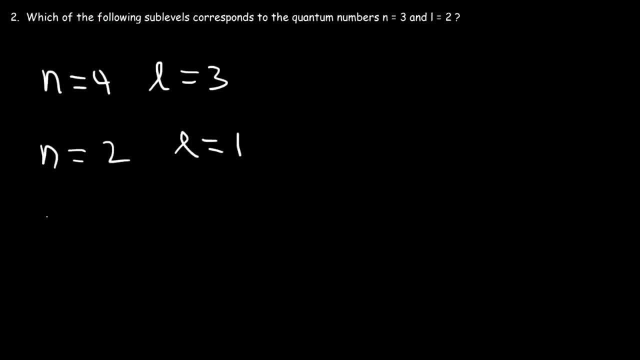 Let's say, when N is 2 and L is 1. And when N is 5 and L is 2. And also when N is 3 and L is 0. So when L is 0, we're dealing with the S sublevel. So therefore this corresponds to 3S. 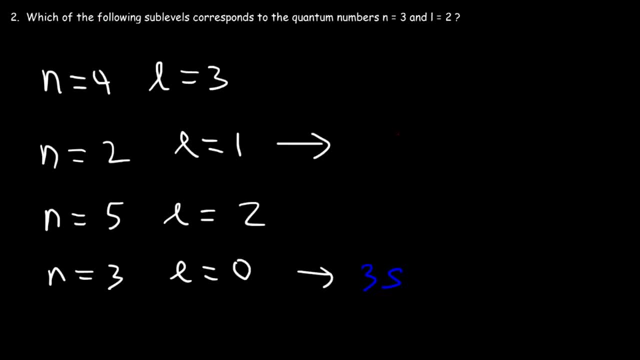 When L is 1, we're dealing with the P sublevel, So this is going to correspond to 2P. The 2 comes from the principal quantum number, N. When L is 2, we have the D sublevel, So this is going to be 5D. 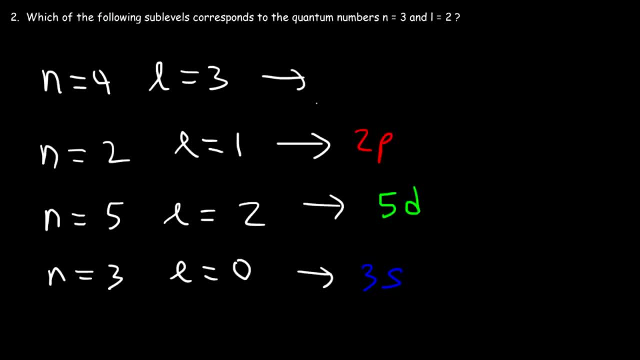 And when L is 3, it corresponds to F. So this is going to be 4F. So hopefully you understand what sublevel corresponds to a particular N and L value. Now let's move on to number 3.. Which of the following sublevels does not exist? 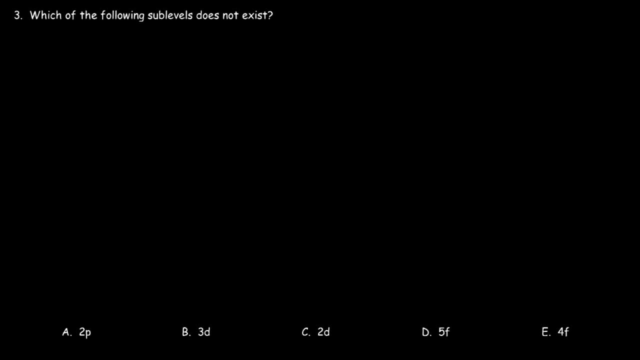 Is it 2P, 3D, 2D, 5F or 4F? Well, let's go through the list. As we said before, in the first energy level there's only one sublevel, And that is the 1S sublevel. 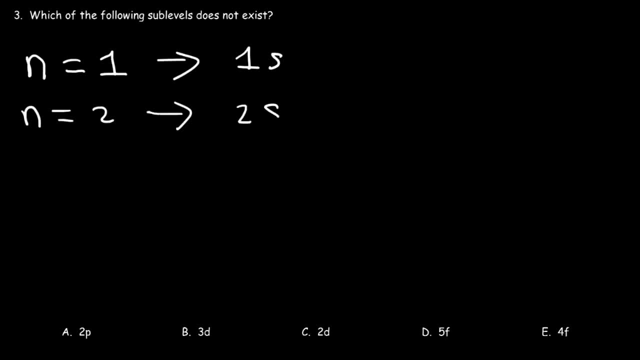 In the second energy level there's two sublevels: 2S and 2P. In the third energy level we have 3S, 3P, 3D. There's three sublevels. In the fourth one it's going to be 4S, 4P, 4D and 4F. 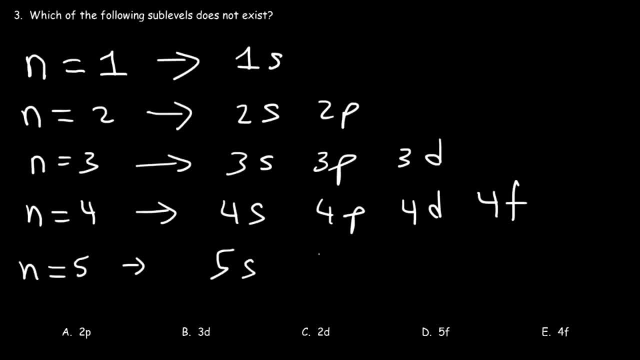 And the fifth one also has 5.. 5S, 5P, 5D, 5F And I believe the next one's either like 5G or 5H, But for the case of this problem we do have 2P. 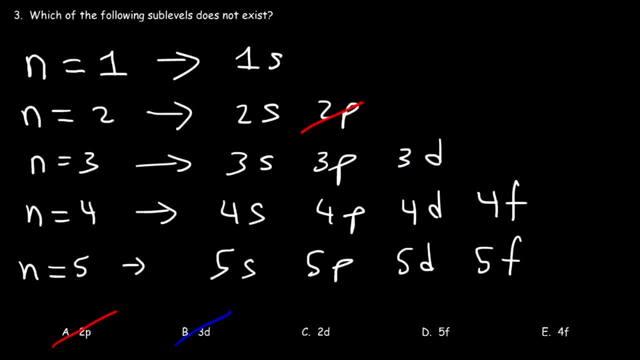 So 2P exists, 3D also exists, 5F exists as well, And the same is true for 4F. So the answer is 2D. There's no D sublevel in the second energy level, So C is the answer. 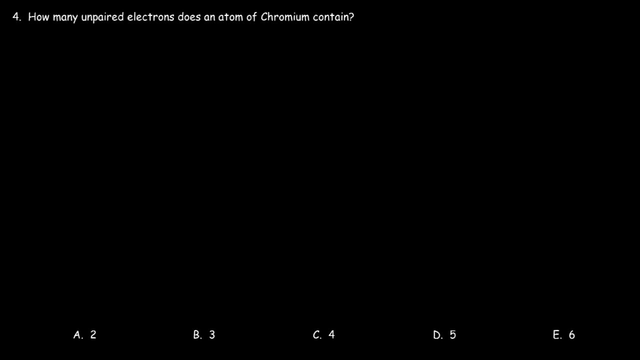 Now let's move on to number 4.. How many unpaired electrons does an atom of chromium contain? In order to find the answer, we need to write the electron configuration of chromium And at the same time draw the orbital diagram. So chromium has 24 electrons. 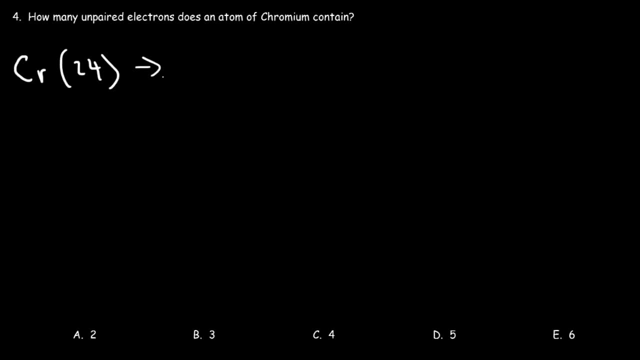 You can find this based on the atomic number in the periodic table. An atom has an equal number of protons and electrons. Now if you write the configuration, you might think it's supposed to be like this: 1S2, 2S2, 2P6, 3S2, 3P6, 4S2, 3D4. 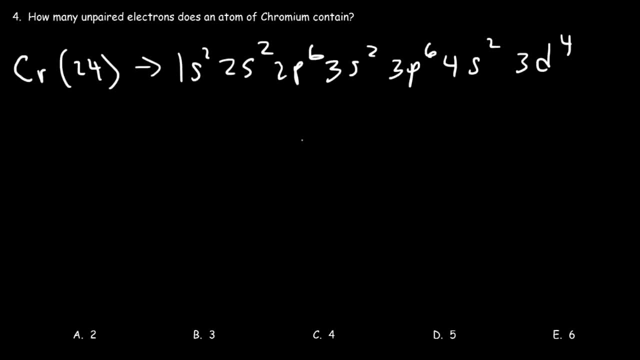 If you add up the exponents, this will give you 24.. However, chromium is one of those exceptions, And it turns out that one of the S electrons jumps to the 3D sublevel. So instead, the configuration is everything you see here but 4S1, 3D5.. 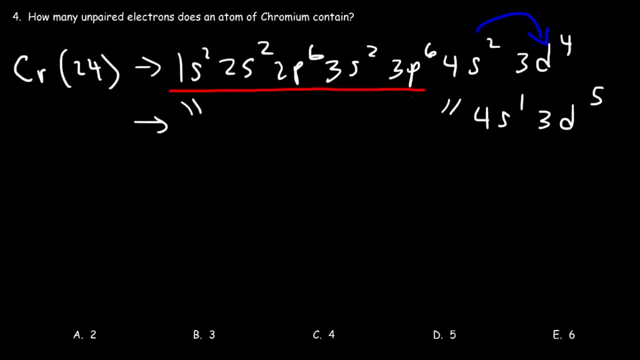 Now, everything from 1S2 to 3P6 will be completely filled, So I'm going to focus on the last two sublevels, That is, the 4S sublevel and 3P6.. The 3D sublevel. 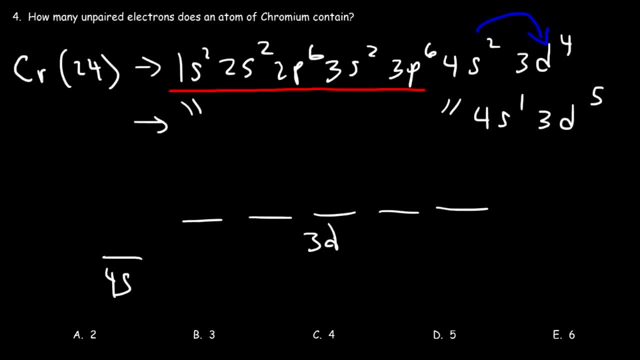 S has one orbital and D has five orbitals. Now, if you were working with this configuration, you would fill up the 4S sublevel and the 3D sublevel, So you might pick 4 as your answer. It might appear that chromium has four unpaired electrons. 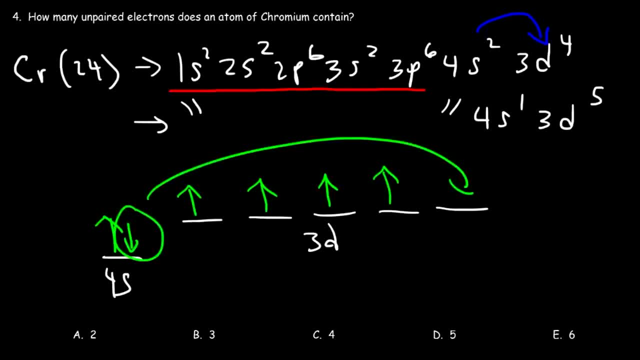 However, when this electron jumps to the 3D sublevel, the situation is going to be different. It turns out that chromium, which is 4S1, 3D5, has a total of six unpaired electrons, And so E is the answer. 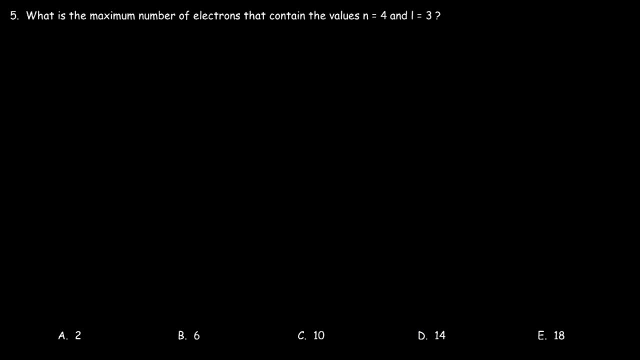 Now let's move on to number five. What is the maximum number of electrons that contain the values N equal 4 and L equal 3?? So if we're given N and L, how can we calculate the number of electrons? The first thing I would do is write the designation of the sublevel that corresponds to those numbers. 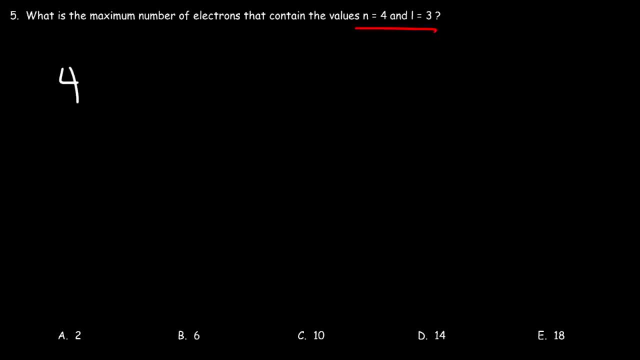 So N is 4.. And when L is 3, does it correlate to the S sublevel, P, D or F? So remember, for S, L is 0.. For P, L is 1.. For the D sublevel, L is 2.. 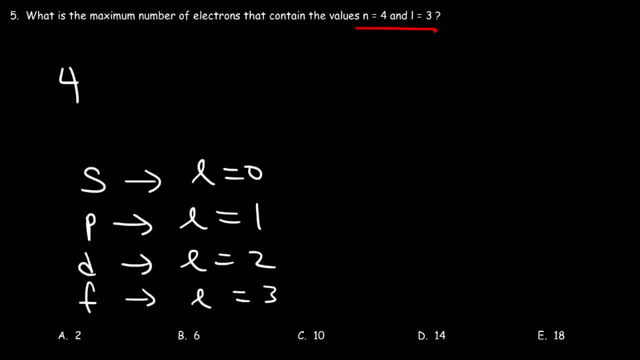 But for F, L is 3.. So since L is 3, we're dealing with the 4F sublevel. Now, how many electrons can be in the F sublevel? S can hold two electrons, P can hold six. 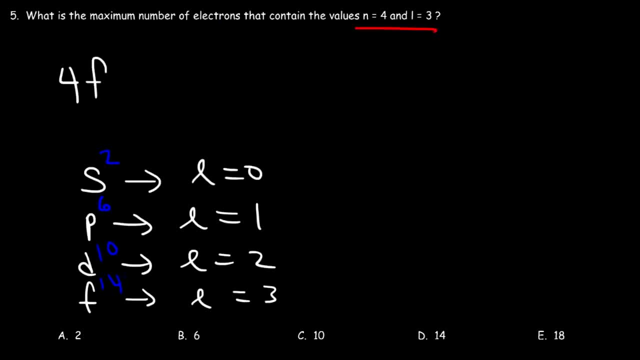 D can hold 10.. F can hold a maximum of 14.. So you can have up to 14 electrons in the 4F sublevel. So D is the right answer for this problem. Okay, let's work on this one, number six. How many paired electrons are in an atom of chlorine? Chlorine has an atomic number of 17 and an average atomic mass of 35.45.. So we can easily find the answer if we write the orbital diagram of chlorine. So what we're going to do is fill up the energy levels until we get to a number 17.. 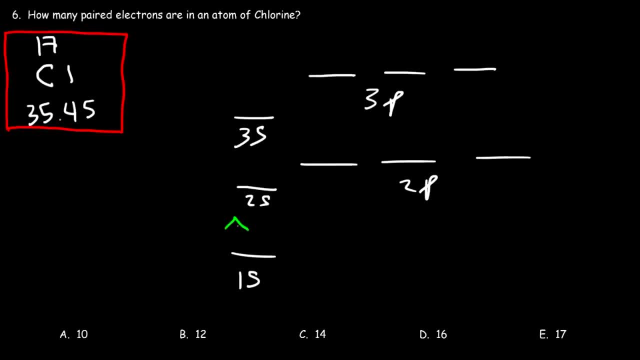 And we could add more if we need it. So we're going to put 2 in the first sublevel, another 2 in the second, So that's 4.. And right now we have 7.. And then this is 10,, 12,, 13,, 14,, 15,, 16,, 17.. 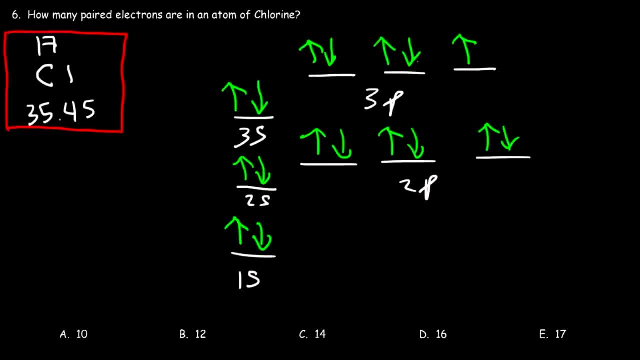 So the electron configuration of chlorine is 1s2, 2s2, 2p6,, 3s2, 3p5.. So we only have 1 unpaired electron, Which means the other 16 must be paired. 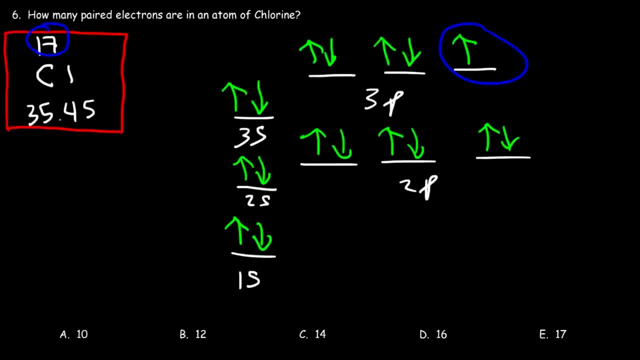 Because we have a total of 17 electrons, Or you can count them: 2,, 4,, 6,, 8,, 10,, 12,, 14,, 16.. So we have 16 paired electrons and 1 unpaired electron. 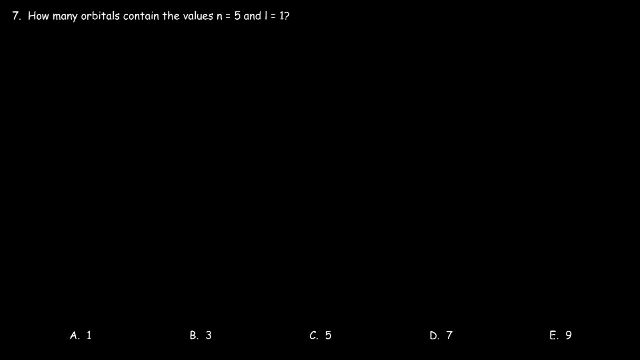 So D is the answer. Number seven: How many orbitals contain the values n equal 5 and l equal 1?? So that's an interesting question. How can we find the answer? So what sublevel does this correspond to? If you're given an n and l value, you could find a sublevel. 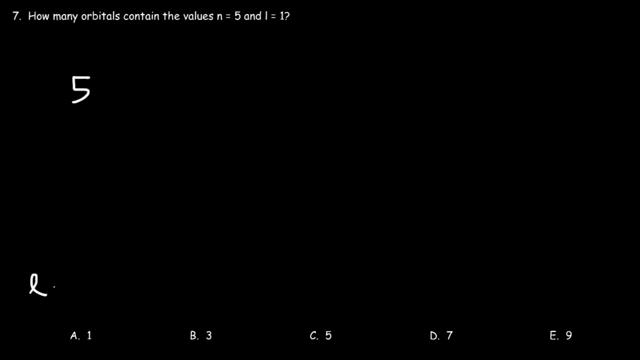 So we're dealing with the fifth energy level. And keep in mind, when l is 0,, we're dealing with the s sublevel, But when l is 1,, we're dealing with the p sublevel. So we're dealing with the 5p sublevel. 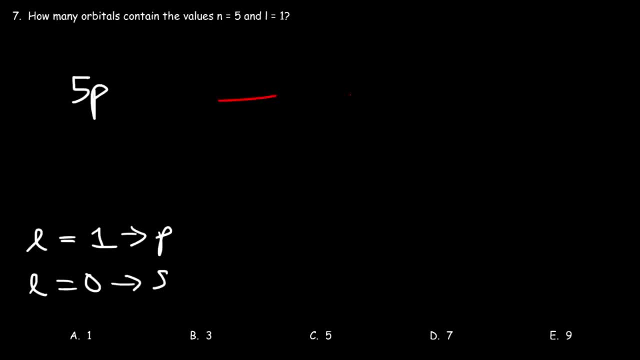 Now, p contains 3 orbitals, s only contains 1.. d contains 5.. So in the 5p sublevel there's only going to be 3 orbitals. So b is the right answer in this problem, Number eight. 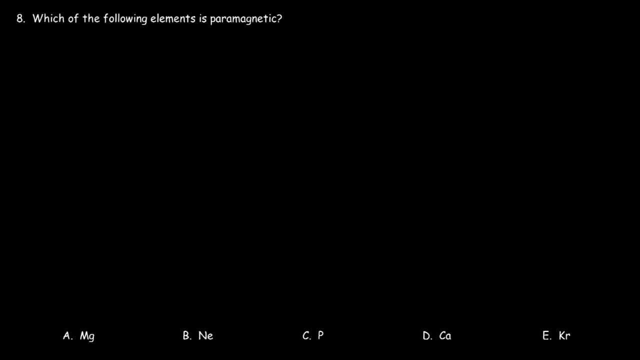 Which of the following elements is paramagnetic? Is it going to be magnesium, neon, phosphorus, calcium or krypton? Number 10.. Now, for an element to be paramagnetic, it has to contain unpaired electrons. So we need to identify which of these elements contain unpaired electrons. 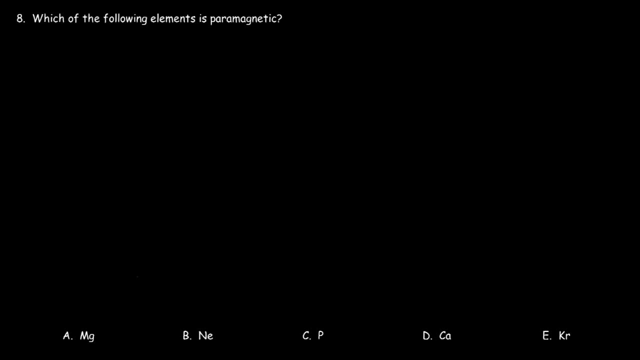 A quick and simple test is to look at the atomic number. Magnesium has an atomic number of 12.. Neon is 10.. Phosphorus is 15.. Calcium is 20. And krypton is 36.. So, looking at these numbers, what do you see? 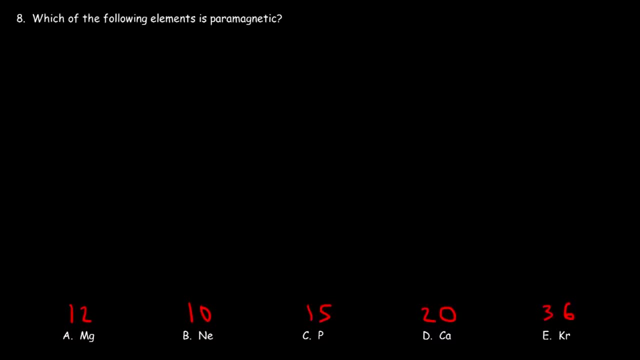 Is there a number that stands out? Notice that four numbers are even. One number is odd. When you have an odd number of electrons, at least one of those electrons has to be unpaired. Three might be unpaired, It might be five. 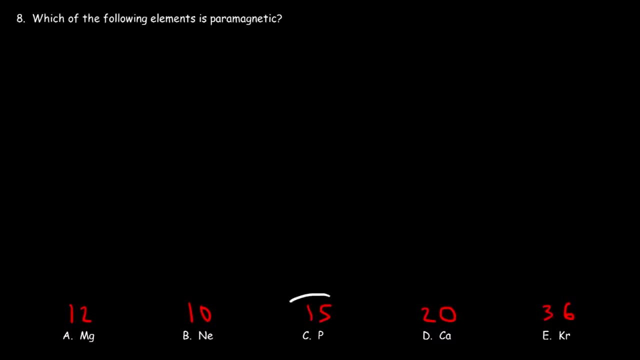 But at least one of them has to be unpaired. So we know for a certain, or rather for certainty, that phosphorus is going to be paramagnetic Because it has an odd number of electrons. Now for the other four, it may or may not be paramagnetic. 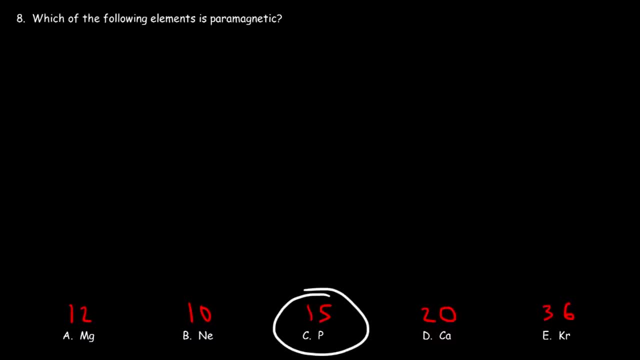 They may or may not contain unpaired electrons, So we have to check to be sure. So let's start with magnesium. Actually, let's start with neon, because it has the lowest number of electrons. So neon has 10 electrons. So this is 2,, 4,, 7, and 10.. 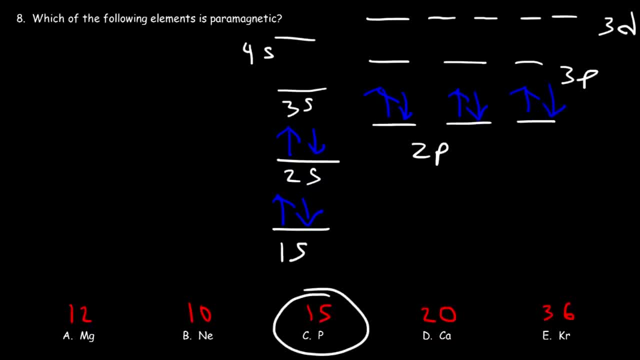 So this is the orbital diagram representation of neon. As you can see, neon is completely paired. It doesn't have any unpaired electrons. So neon is going to be diamagnetic. Now magnesium has 10 electrons, That's 12.. So we only have to add two more. 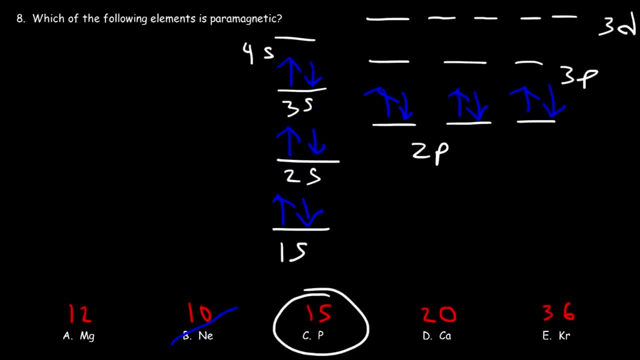 So that's the configuration for magnesium. It's 1s2, 2s2, 2p6, 3s2.. So it's diamagnetic. It doesn't have any unpaired electrons. Now let's move on to calcium. 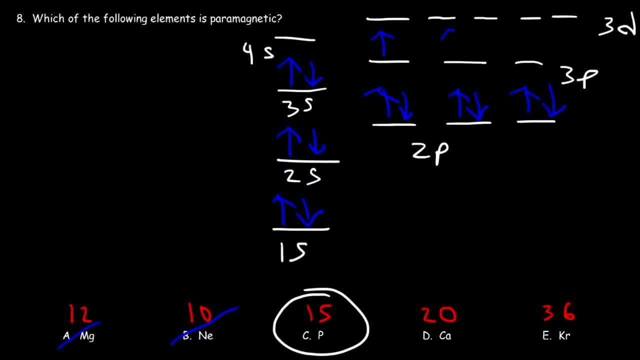 So we need to get up to 20.. So right now we have 12., Now we have 15. And then 18. And now we have 20.. So that's the picture for calcium. So it's diamagnetic as well. 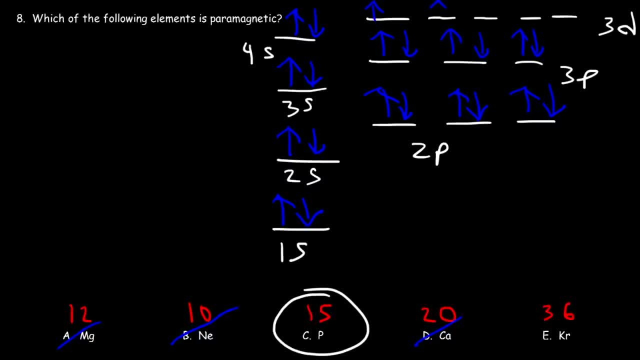 Now we need to get up to 36.. So right now we have 25.. And now we have a total of 30. After the 3d sublevel comes 4p. So now we have 33. And then 36.. 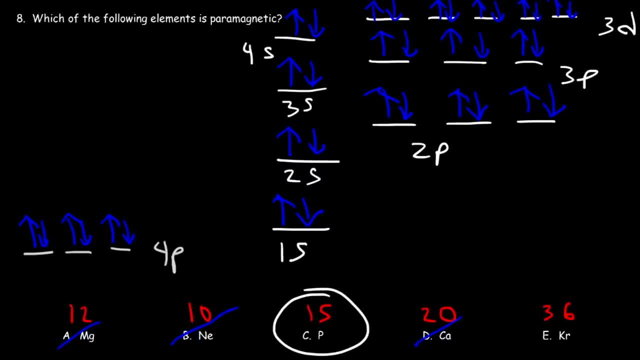 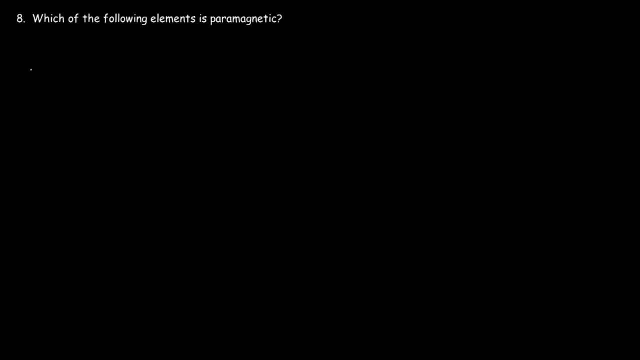 So krypton is completely paired. It doesn't have any unpaired electrons, So it's diamagnetic as well. Now let's draw the orbital diagram for phosphorus. Let's see how many unpaired electrons it has. So this is 1s, 2s, 2p, 3s and 3p. 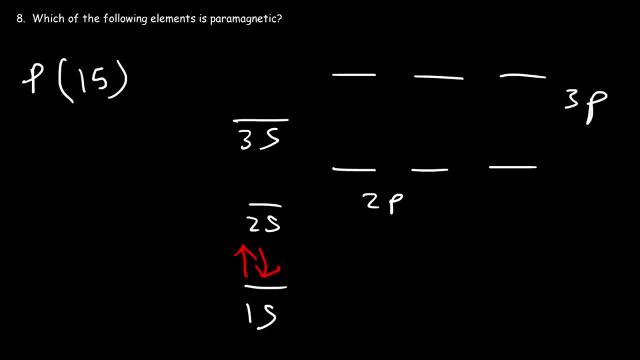 So let's draw arrows until we reach a total of 15.. So we have 2, 4.. 4,, 7,, 10, and 12.. And according to Hund's rule, we need to add one electron at a time when dealing with degenerate. 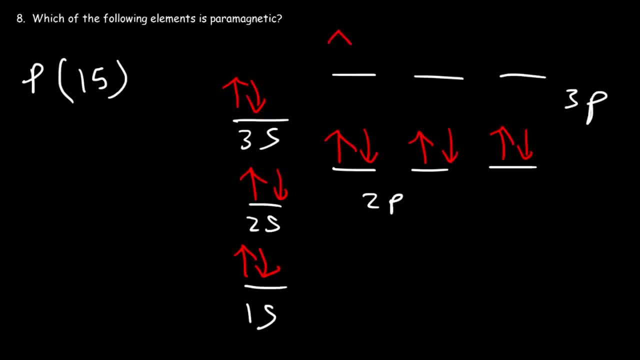 orbitals or orbitals of equal energy. So this is going to be 13,, 14,, 15.. So out of the 15 electrons, 3 electrons are unpaired. I'm going to put up for unpaired And the other 12 are unpaired. 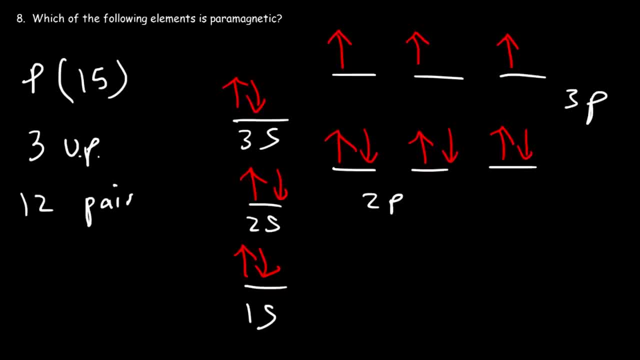 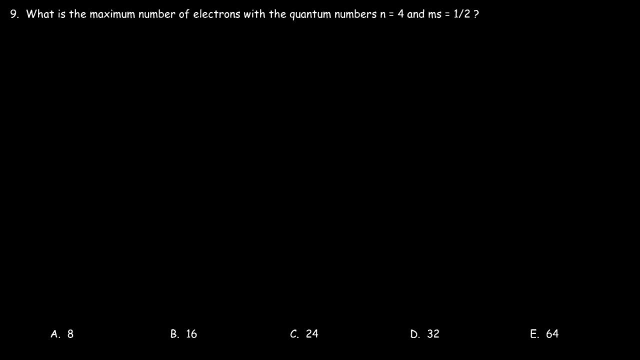 And the other 12 are paired electrons. So based on these three unpaired electrons, we can say that phosphorus is paramagnetic. It's weakly attracted to an external magnetic field. Now what about this question? What is the maximum number of electrons with the quantum numbers? n equals 4 and ms, the electron spin is positive 1 half. 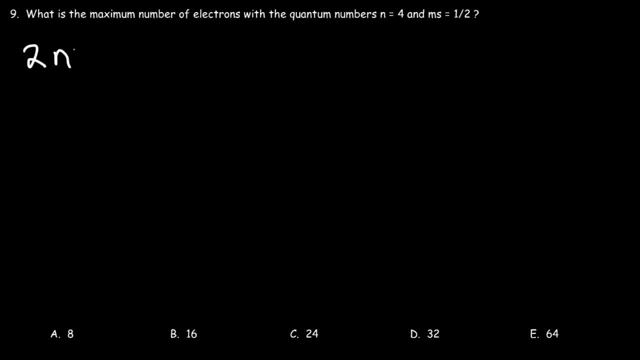 Well, the maximum number of electrons in a certain energy level is 2n squared. So when n is 4, this is going to be 2 times 4 squared. 4 squared is 16, times 2 is 32.. 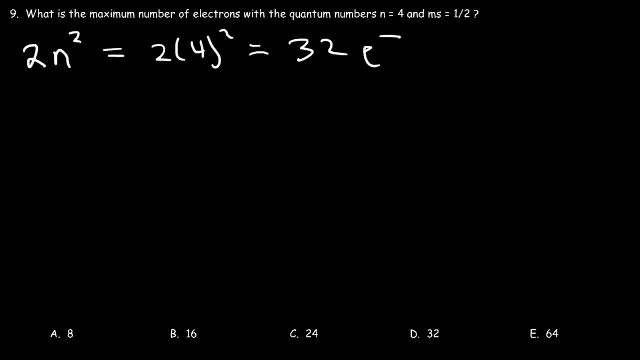 So there's 32 electrons that can be in the fourth energy level. Now, how many of these electrons will have a spin of plus 1 half? Now, within an orbital there's two potential spins. It's either up or down. So, out of these three unpaired electrons, how many of these electrons will have a spin of plus 1 half? 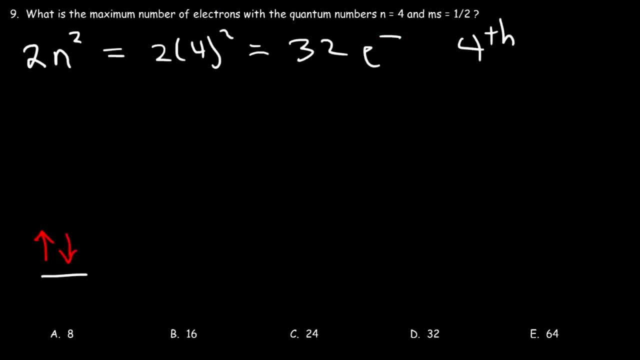 So out of these 32 electrons, half of them will contain an up arrow and the other half will have a down arrow, So 16 will have a spin of plus 1 half and the other 16 will have a spin of negative 1 half. 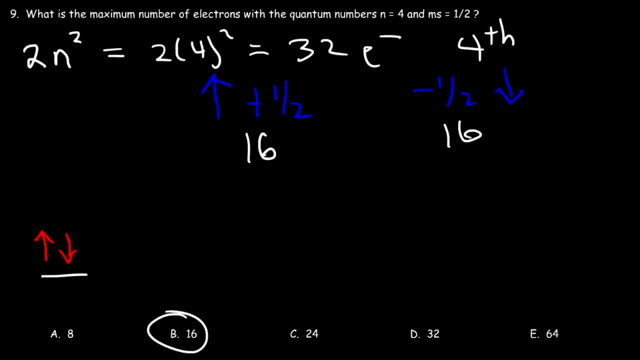 So, therefore, the answer should be 16.. Now, if you want to see this for yourself, you can draw it out if you want to. So, in the fourth energy level, we have 4s, 4p, 4d and 4f. 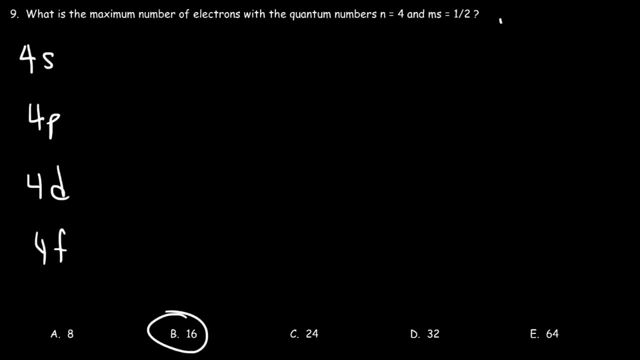 So keep in mind, the number of sub-levels is equal to the energy level. So if you're dealing with the fourth energy level, there are 4 sub-levels. If you're dealing with the third energy level, there are 3 sub-levels. 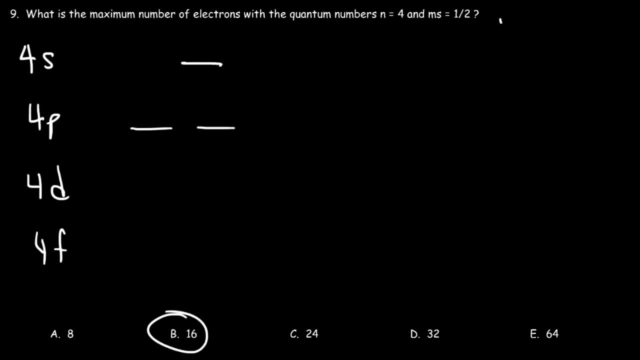 s has 1 orbital, p has 3.. d has 5 orbitals, f has 7 orbitals. Now, because this is a three-dimensional system, now because the electron spin is positive 1 half and not negative 1 half, 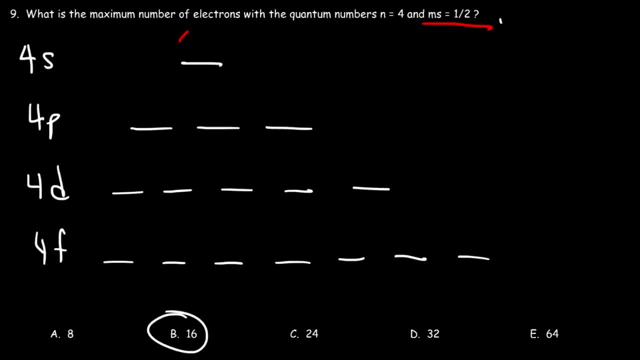 we only want to draw the arrows that are facing upward. So in a 4s orbital there's only one arrow that has a spin of plus 1 half. In the 4p sub-level there's 3 of such electrons. 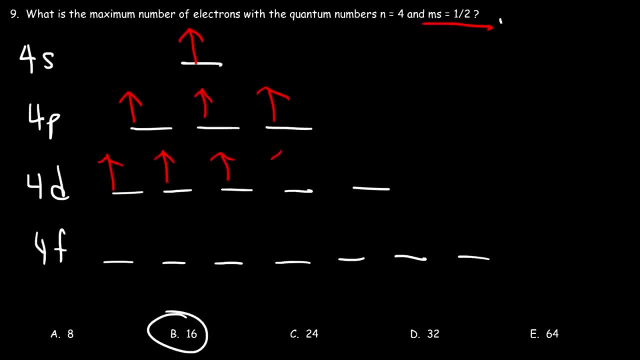 In 4d there's going to be 5. And in 4f there's going to be 7 that have a spin of plus 1 half. So now let's add up these numbers, So we have 1,, 3,, 5, and 7.. 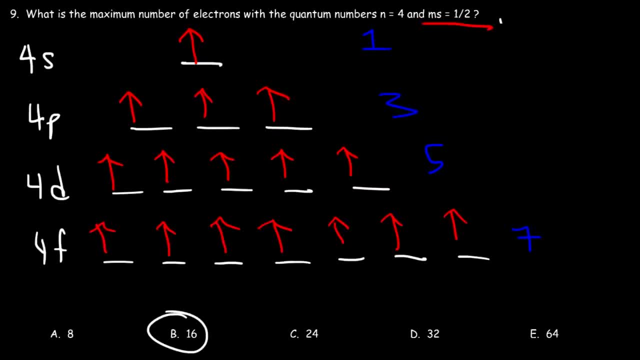 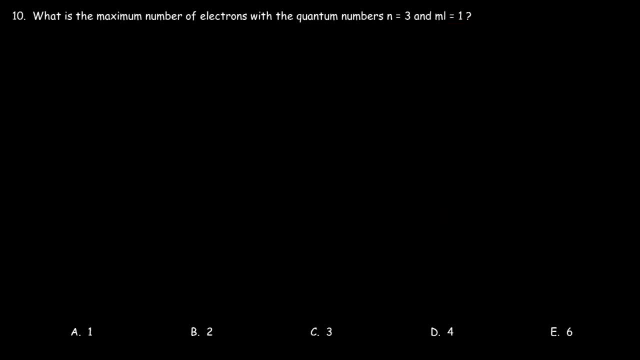 1 plus 3 is 4.. 4 plus 5 is 9.. 9 plus 7 is 16.. So b is the right answer, Number 10.. What is the maximum number of electrons with the quantum numbers n equals 3 and ml equals 1?? 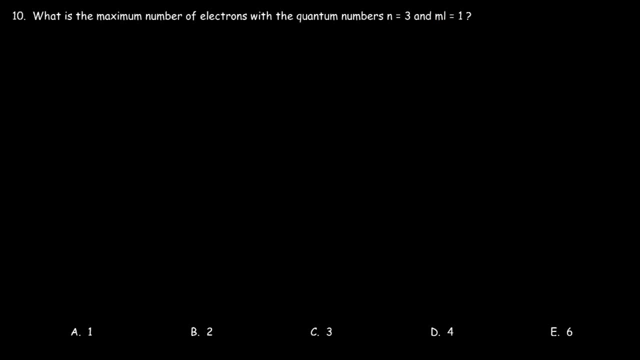 So we're given examples where we had n and l, Where we had n and l, n and ms, and now n and ml, The energy level and the magnetic quantum number. So how can we do this, How can we find the maximum number of electrons with these two quantum numbers? 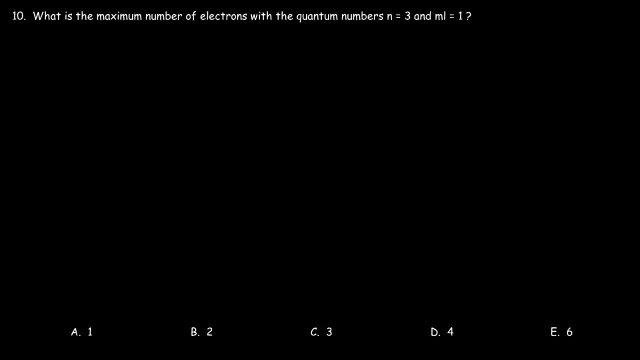 If you're not sure, draw it out. In the third energy level there are three sub-levels: 3s, 3p and 3d. Now s only has one orbital, p has three orbitals And d has five orbitals. 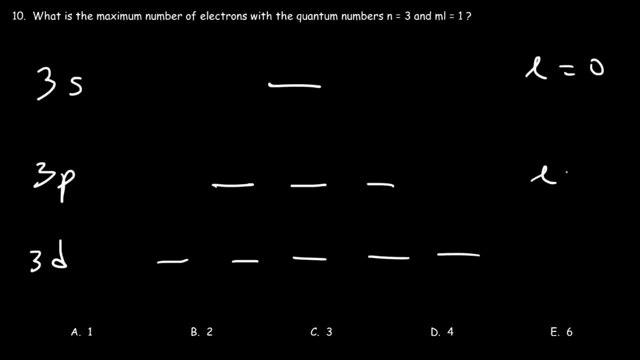 Now for the s sub-level, l is 0.. For the p sub-level, l is 1.. And for the d sub-level, l is 2.. Now it's important to understand that ml varies between negative l and l. So in the case of the s orbital, l is 0, so ml can only be 0.. 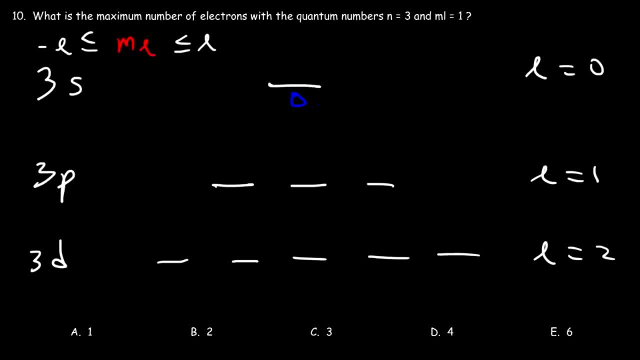 Now for the p sub-level, l is 0.. So ml can only be 0.. l is 1,, so ml can be from negative 1 to 1.. And for the d sub-level, l is 2,, so ml can vary between negative 2 and 2.. 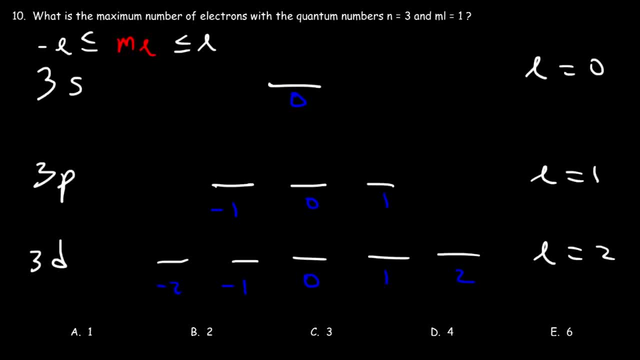 Now our goal is to focus on an ml value of 1.. And there's two orbitals that have it. There's one in the 3p sub-level and there's one in the 3d sub-level. Now we can only put two electrons in each of these orbitals. 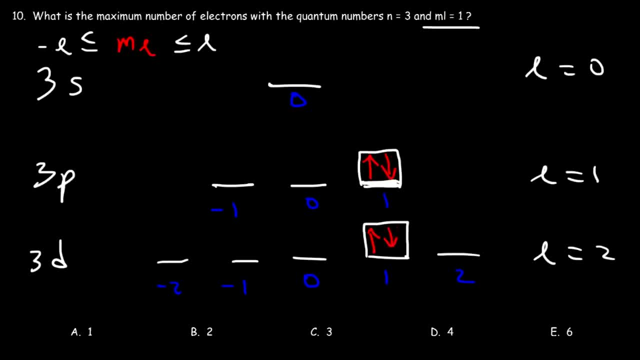 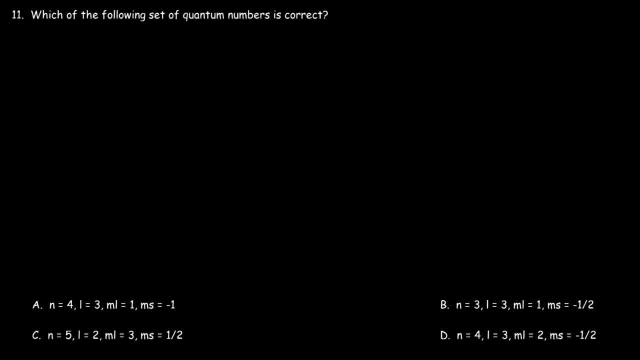 So therefore, there are four electrons that can have the n equal 3 value with an ml value of 1.. So therefore, d is the right answer in this problem, Number 11.. Which of the following set of quantum numbers is correct: 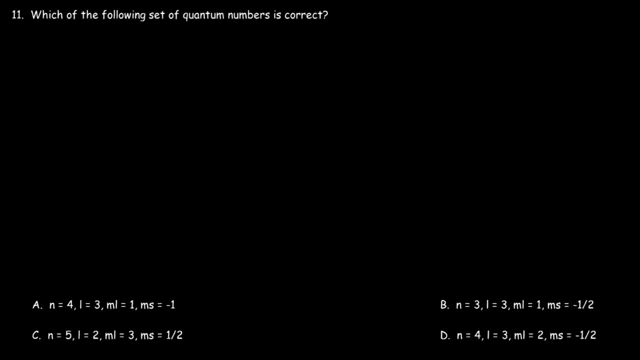 So how can we find the answer to this? Well, the first thing we should compare are n and l. You need to understand that l has to be less than or equal to n minus 1.. So if n is 4, l can be anything from 0 to 3.. 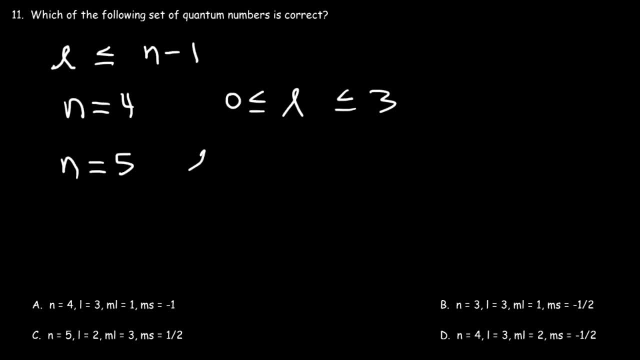 But it can't be 4.. So if n is 5,, l has to be 4 or less. So if n is 5, l can't be 5.. If n is 6,, l has to be 5 or less. 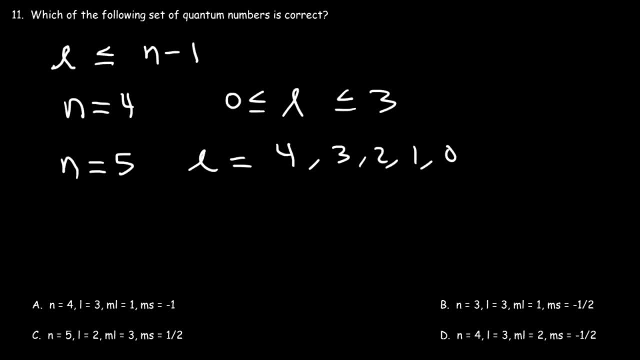 l can't be 6 or 7.. So, looking at a, if we compare the n and l values, so when n is 4, l is 3, that's fine. Looking at b, when n is 3, l can be 3.. 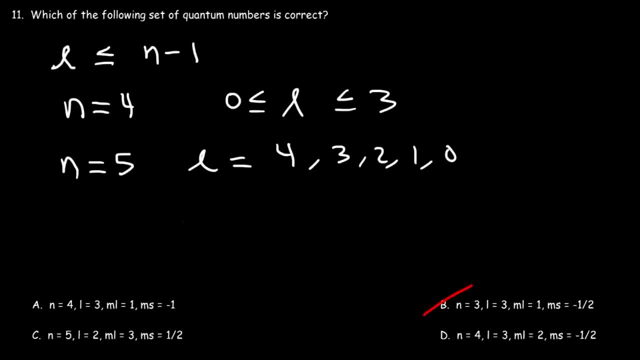 It has to be 2 or less, So we could get rid of answer choice b. Looking at c, n is greater than l, so that's fine. And for d, n is greater than l, So make sure that's always the case. 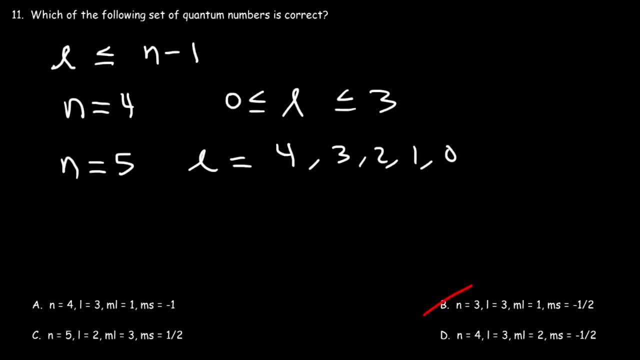 l can't be equal to n or greater than n. n has to be greater than l. So that's the first thing we're going to look for Now. the next thing we need to do is compare l and ml. So ml is always going to be between negative l and l. 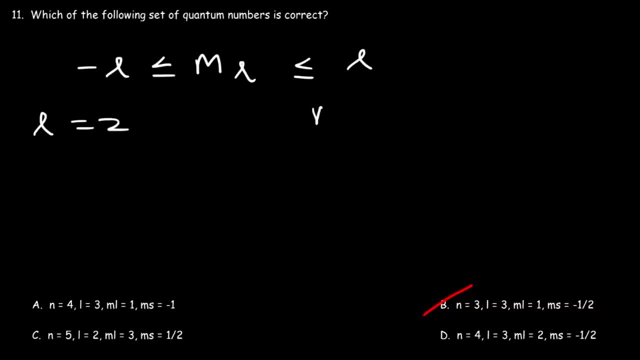 So let's say if l is 2.. ml has to be between negative 2 and 2.. So, ignoring the negative sign, ml should not be larger than l. It should be equal to or less than that number. So if l is 3,, 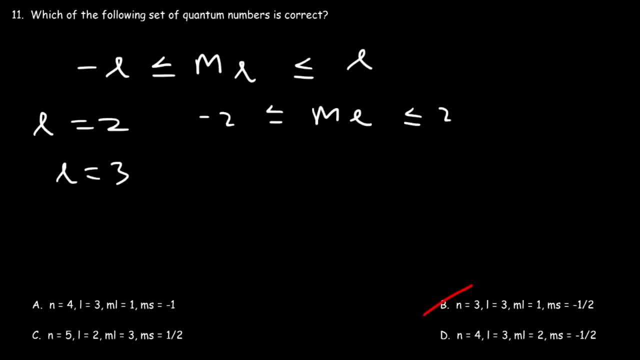 ml should not be 4 or 5. It could be between negative 3 and 3. It can't be negative 4. It can't be 7. It has to be within that range. So, looking at a comparing l and ml, ml is less than l. 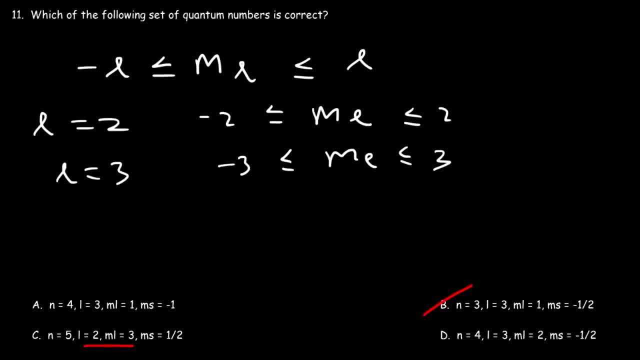 So a is okay. Looking at c, ml is greater than l. That's not good. If l is 2, ml has to be between negative 2 and 2. It can't be 3. So we can eliminate answer choice c. 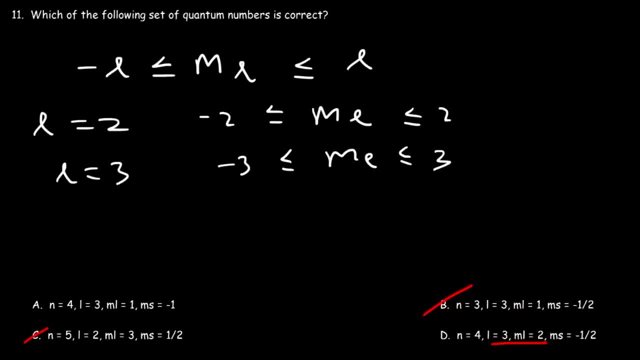 Looking at d, l is greater than ml, So that's okay. Now the last thing that we need to consider is the electron spin, which can only be one of two values. It can be positive or negative- 1 half, So it has to be a fraction. 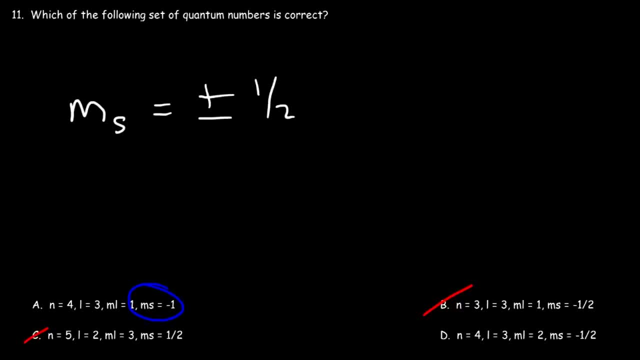 If you don't see a fraction, then it's not correct. So looking at a ms is negative 1. It's not a fraction, So a is eliminated. And looking at d, we do have a fraction, So d is the one that is correct. 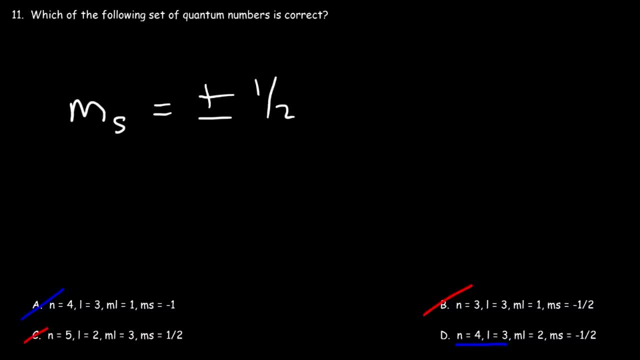 n is greater than l And l is greater than ml, And ms is a fraction, either 1 half or negative 1 half. So this is the right answer. Now let's move on to number 12.. How many orbitals are located in the n equal 4 energy level? 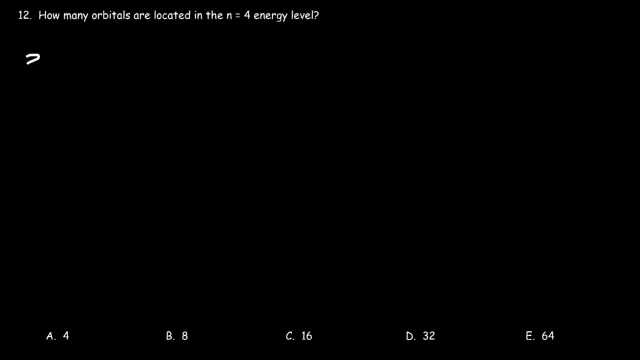 Now recall that the max number of electrons is equal to 2n squared, if you're only dealing with the energy level and those sublevels or anything other than that. Now within an orbital you can have two electrons. So the maximum number of orbitals is half of the maximum number of electrons. 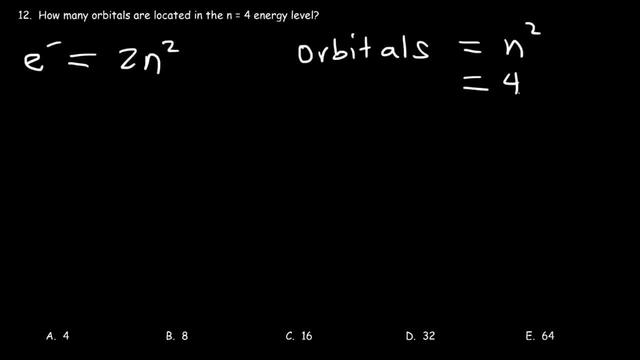 It has to be equal to n squared, So therefore we should expect an answer of 4 squared, which is 16, which means c should be the right answer. Now let's confirm it. In the 4th energy level there are 4 sublevels. 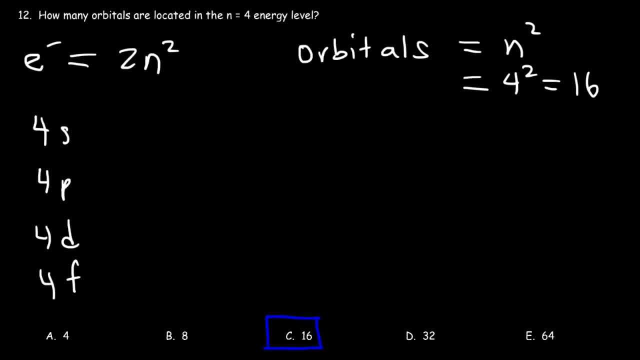 4s, 4p, 4d and 4f. Now s has 1 orbital, p has 3.. d has 5. And f has 7 orbitals. So we're going to add up the numbers 1,, 3,, 5, and 7,. 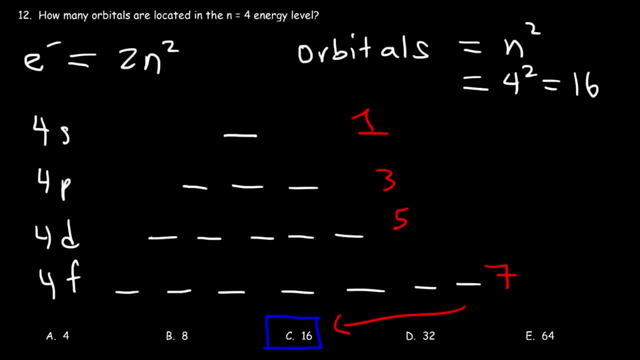 which we know to be 16.. So c is the right answer. So the maximum number of orbitals in an energy level is simply equal to n squared, And the maximum number of electrons in an energy level is 2n squared. Now what about this one? 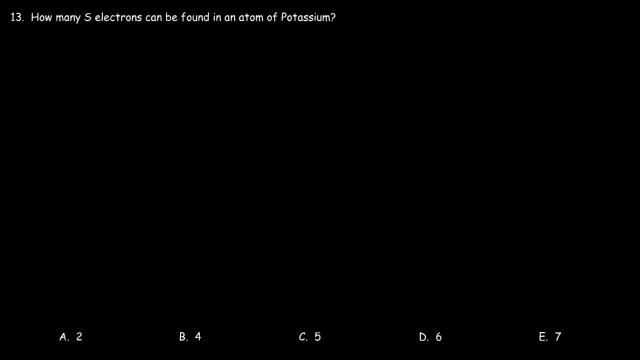 How can we find the number of s electrons that can be found in an atom of potassium? So potassium has an atomic number of 19.. So what I recommend doing is writing the orbital diagram of potassium. Or you can write the electron configuration, But I think drawing the orbital diagram is easier. 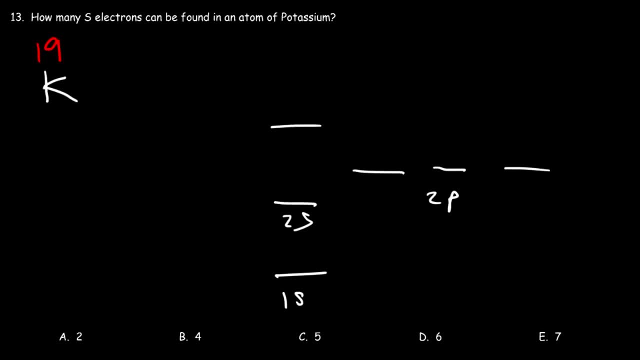 because all you've got to do is fill it up until you reach a total of 19.. So let's fill up the lower energy levels first, based on Off-Bos principle. So we have 2,, 4,, 7,, 10, and 11.. 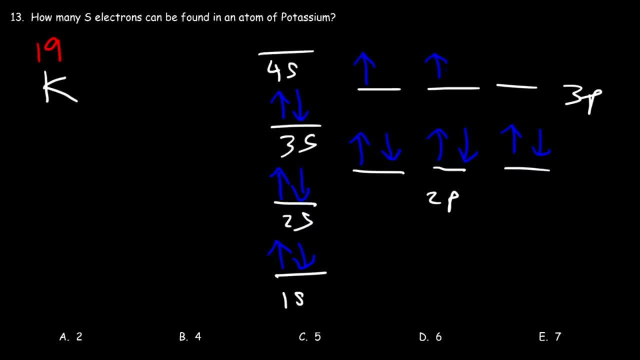 12, 15,, 18,, 19,. well, that's 18 and then 19.. So we have 1 unpaired electron. So the electron configuration of potassium is 1s2, 2s2, 2p6, 3s2, 3p6, 4s1. 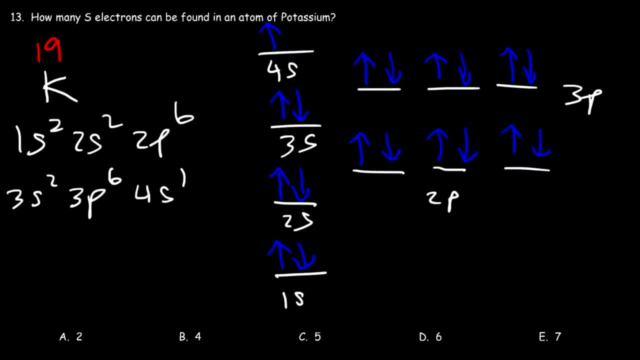 So if you want to find the number of s electrons using the orbital diagram, just count the electrons that have an s on it. So this is 2, 4, 6, 7.. Or you can see it here: 2, 4, 6, 7.. 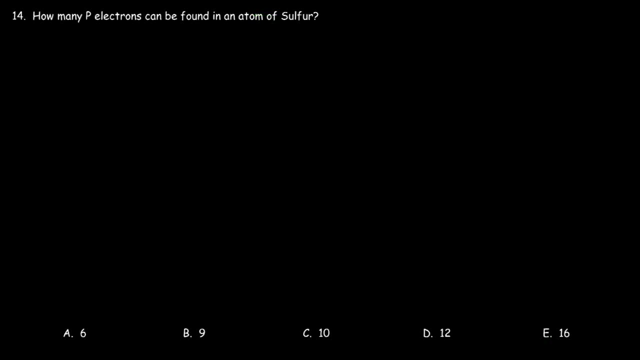 So e is the right answer. So now that you know how to do the last problem, let's try another similar problem: How many p electrons can be found in an atom of sulfur? So sulfur has an atomic number of 16.. So let's try the orbital diagram of sulfur. 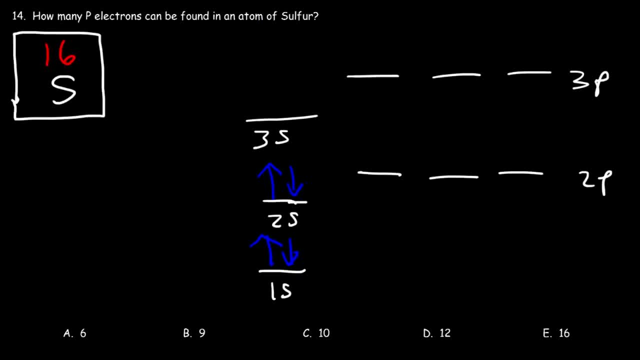 So we have 2,, 4,, 7,, 10,, 12,, 13,, 14,, 15.. 13,, 14,, 15,, 16.. So sulfur is paramagnetic because it has 2 unpaired electrons. 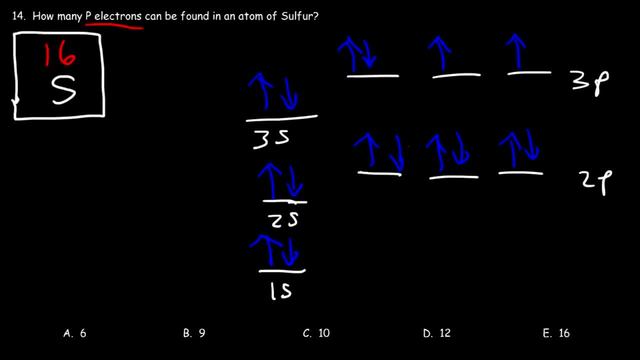 Now our goal is to calculate the number of p electrons. So this is 2,, 4,, 6,, 8,, 9,, 10.. So sulfur has a total of 10 p electrons. Now let's move on to number 15.. 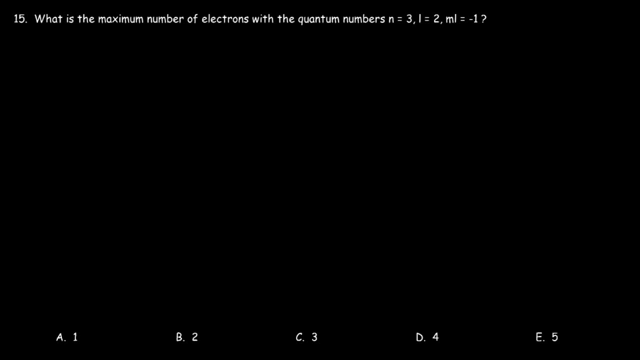 What is the maximum number of electrons With the quantum numbers n equals 3,, l equals 2, and ml equals negative 1.. So if we have all 3 quantum numbers except the electron spin, what is the maximum number of electrons? 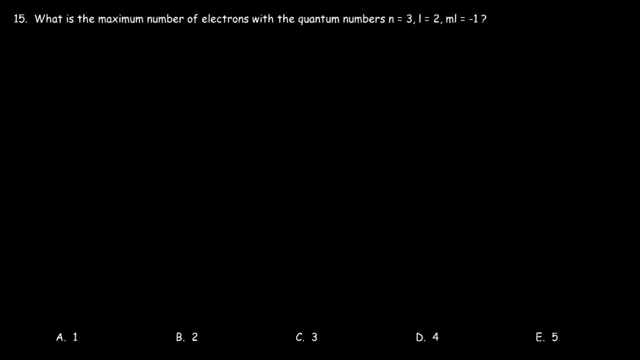 If you have all 3 of these, it can only be 2. Because once you have an ml value, it specifies a single orbital. Now we're dealing with the third energy level, because n is 3.. And when l is 2, we're dealing with the d sub-level. 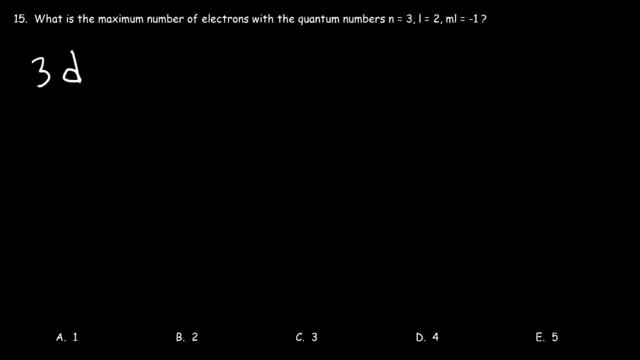 So we're dealing with the 3d sub-level. Keep in mind, when l is 0,, you're dealing with s, When l is 1, it's p, But it's 2 for d. So now, within the 3d sub-level, there are 5 orbitals. 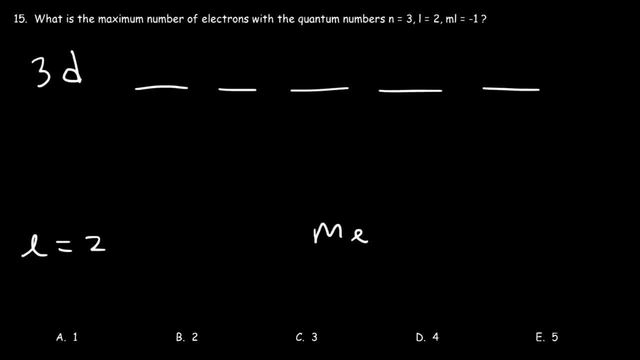 Since l is 2, ml has to vary between negative l and l, So it has to vary between negative 2 and 2.. So this has an ml value of negative 2, negative 1,, 0,, 1, and 2.. 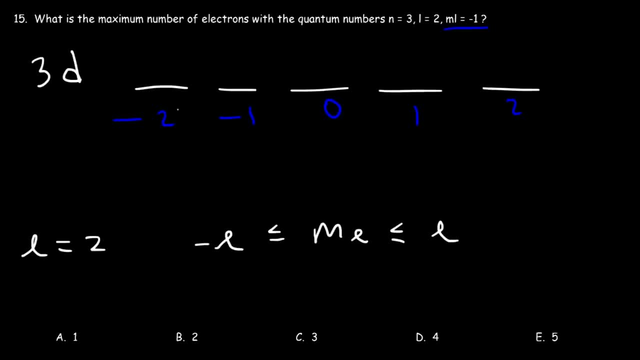 Now ml is negative 1, so we're focused on this orbital, So that orbital can only hold 2 electrons. And so any time you want to find the maximum number of electrons given n, l and ml, it can only be 2.. 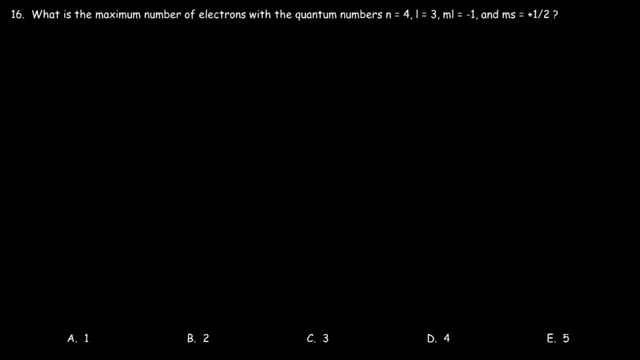 So b is the answer. Now let's try this problem, Number 16.. What is the maximum number of electrons with the quantum numbers? n equals 4,, l equals 3?, ml equals negative 1, and ms equals plus 1 half. 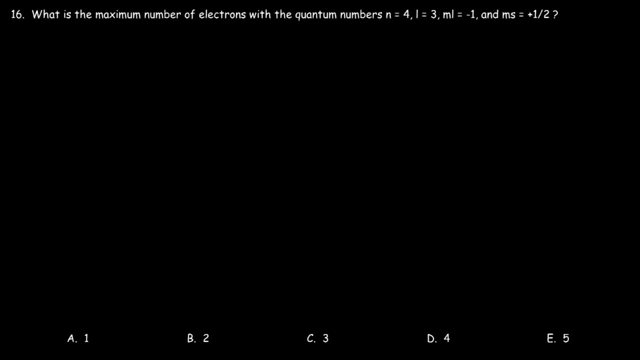 Now, according to Pauli's exclusion principle no 2, electrons can have the same set of 4 quantum numbers. So if these 4 quantum numbers are allowed, then it can only represent 1 single electron. So we have the 4th energy level. 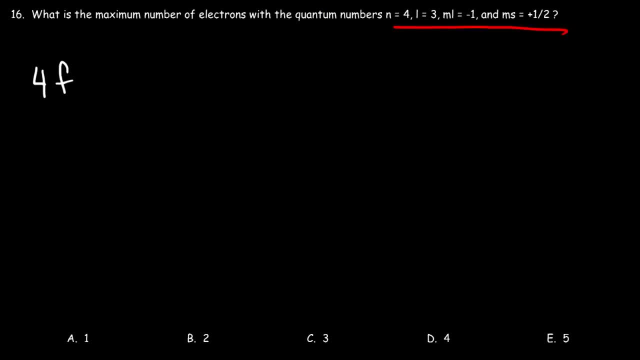 And l is 3 for the f sub-level. So we're dealing with 4f. f has 7 or more electrons. Now, since l is 3, ml is going to vary between negative 3 to positive 3.. Now we need to focus on the orbital with a negative 1 value. 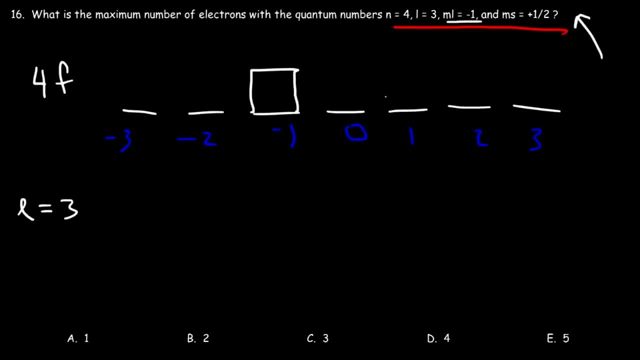 And then within that orbital the electron spin is plus 1 half. So there's only 1 electron that can have those 4 quantum numbers, And it's this electron here. So therefore the answer is a Number 17.. Which of the following elements correspond to the ground state electron configuration? 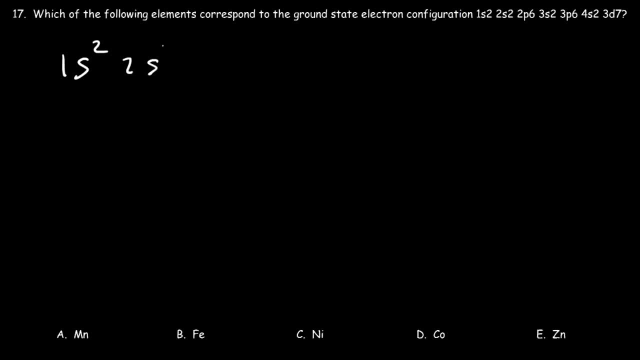 1s2, 2s2, 2p6,, 3s2, 3p6,, 4s2, 3d7.. So if you're dealing with an atom, you can find the atomic number by adding the exponents of the electron configuration. 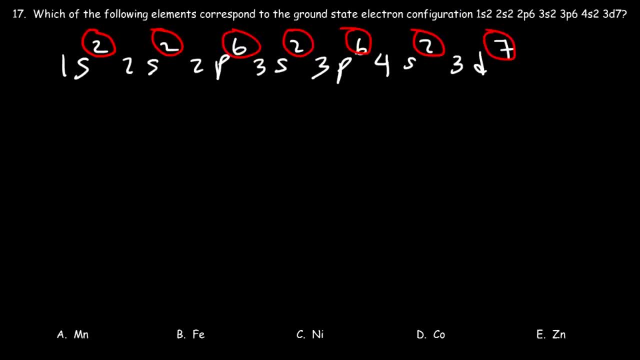 So 2 plus 2 plus 6 is 10.. 2, 6, and 2 is another 10.. That's 20.. Plus 7 is 27.. So what you need to do using the periodic table, is you need to identify which of these elements have an atomic number of 27.. 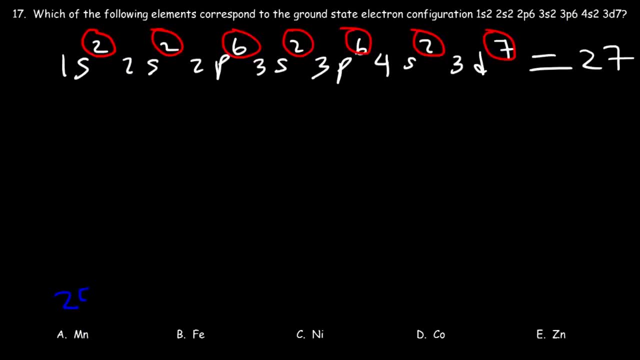 Manganese has an atomic number of 25.. Iron metal has an atomic number of 26.. Nickel is 28.. Cobalt is 27. And zinc is 30. So therefore, this is the electron configuration of cobalt Number 18.. Which of the following elements correspond to the electron configuration argon 4s2,, 3d10, 4p3?. So how can we find the answer? All we need to do is find the atomic number that's associated with this electron configuration and match it with the answers. 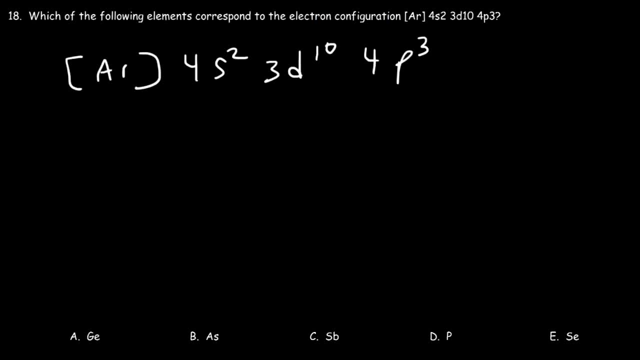 Germanium has an atomic number of 32.. Arsenic has an atomic number of 33.. Antimony is 51. Phosphorus is 15. And selenium is 34.. Now, argon has an atomic number of 18.. 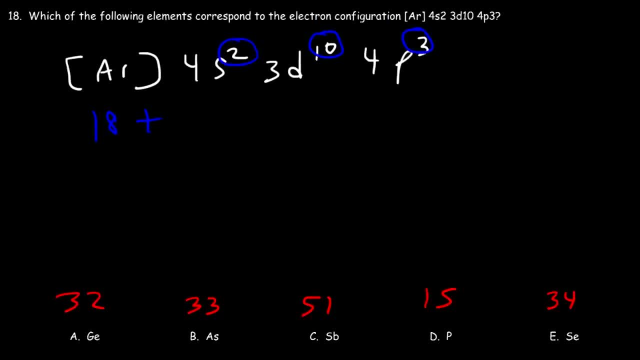 And then add the exponents, So that's plus 2 plus 10 plus 3.. So 18 plus 2 is 20.. 20 plus 10 is 30.. 30 plus 3 is 33.. So therefore this configuration matches with arsenic. 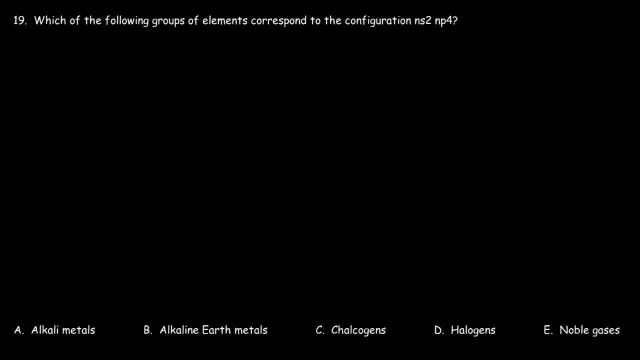 So B is the right answer. Now let's move on to the next problem. Which of the following groups of elements correspond to the configuration ns2 and p4?? Is it going to be the alkali metals, The alkaline earth metals, Chalcogens? 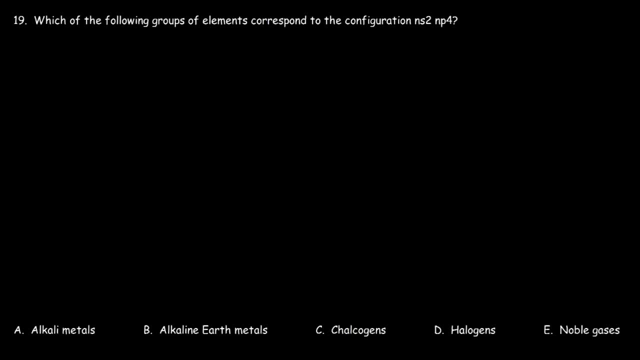 Halogens, Or the noble gases. Well, let's start with group 1.. So we have elements such as hydrogen, lithium, sodium and potassium. So group 1 represents the alkali metals, with the exception of hydrogen, That's not a metal. 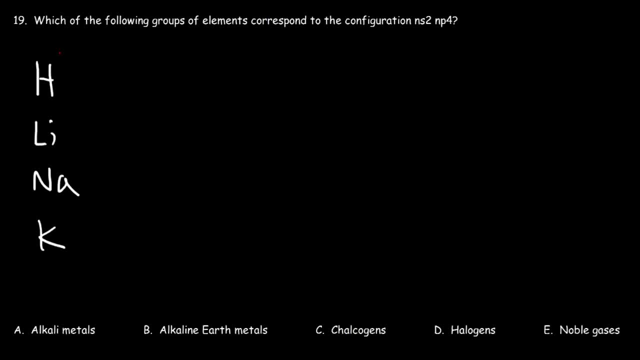 Now, hydrogen has a configuration of 1s1.. Lithium is 1s, I mean it's 2s1.. Sodium ends in 3s1.. Potassium ends in 4s1.. So the alkaline metals has a configuration of ns1.. 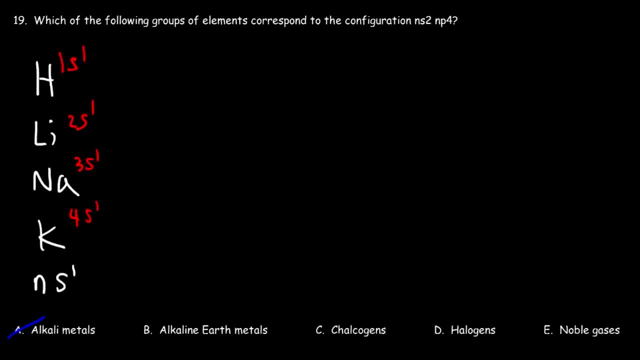 So the answer is not going to be A. Now let's move on to the alkaline earth metals Such as beryllium, magnesium and calcium. Beryllium has a configuration of 2s2.. Magnesium ends in 3s2.. 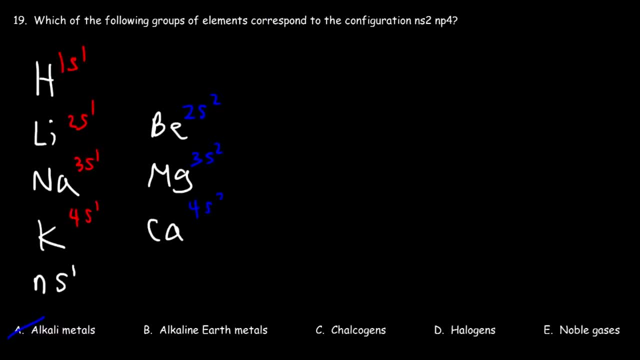 And calcium ends in 4s2.. So the alkaline earth metals group 2a has a configuration ns2.. Now the chalcogens are elements such as oxygen, sulfur, selenium and so forth. Oxygen ends in 2p4.. 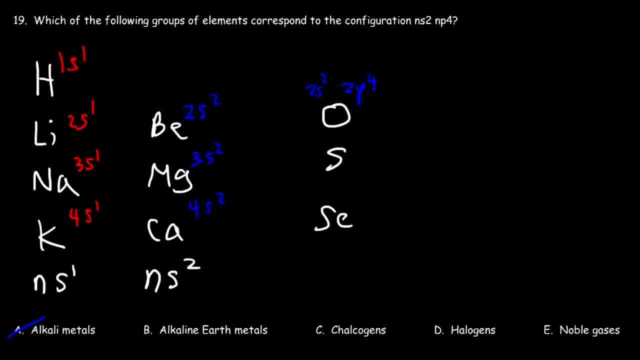 It's 2s2, 2p4.. Sulfur is 3s2, 3p4.. Selenium is 4s2, 4p4.. And of course we're skipping 3d10 for selenium. 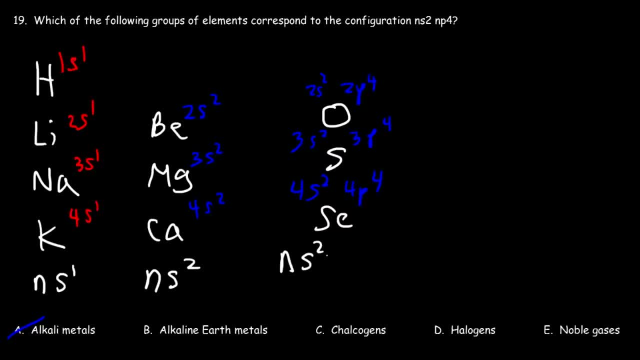 So the chalcogens have the typical configuration ns2, np4. And so C is the answer, The halogens it's ns2, np5. And for the noble gases it's ns2, np6. The exception is helium, because that's just 1s2.. 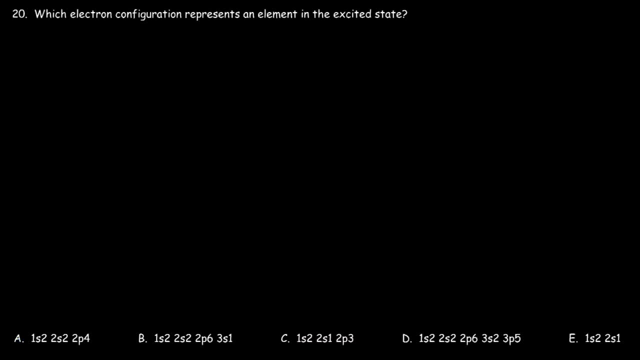 So C is the right answer, Number 20.. Which electron configuration represents an element in the excited state? So we need to see which one skips. If there's any skipping within the electron configuration, it's going to be in the excited state. 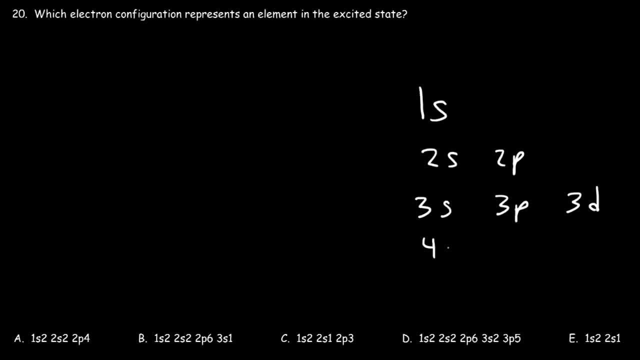 If there's no skipping, then it's a ground state configuration. The S sublevel can hold 2 electrons. P can hold 6.. D can hold 10.. F can hold 14.. So first we need to start with 1s. 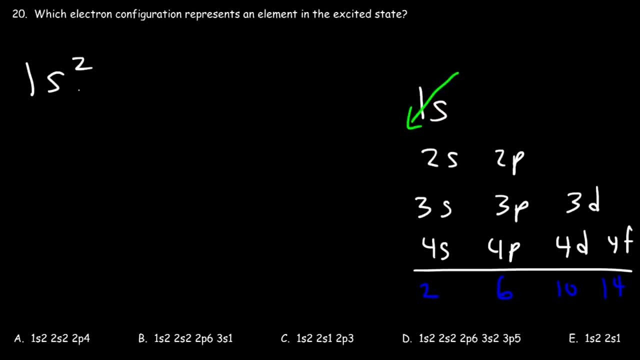 The first configuration is always going to be 1s2.. Which all of them have it. So after the 1s sublevel, we have 2s, So that goes up to 2s2.. Which this one has it. 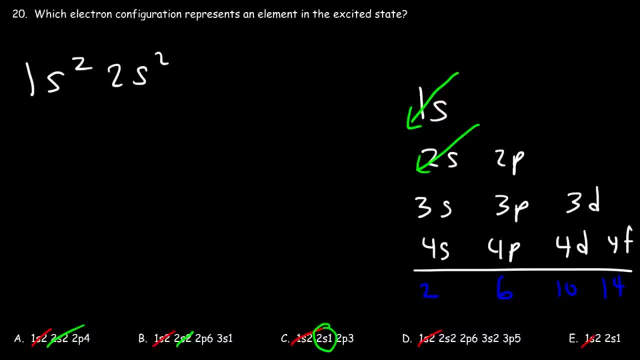 Now notice that this skips. It doesn't go from. it's not completely filled, So we're missing the 2s2 electron. So chances are this is the one that's in the excited state. Everything else goes in order. After 2s, you have 2p and 3s. 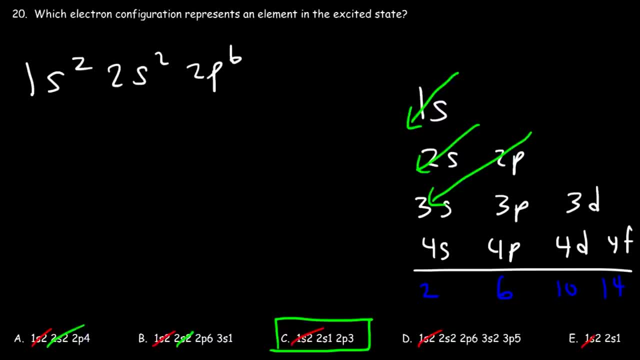 So after 2s2, you have 2p6.. This has 2s2.. This one just ends. After 2s2, you have the 2p sublevel. This has 2p6. And everything else continues in order. 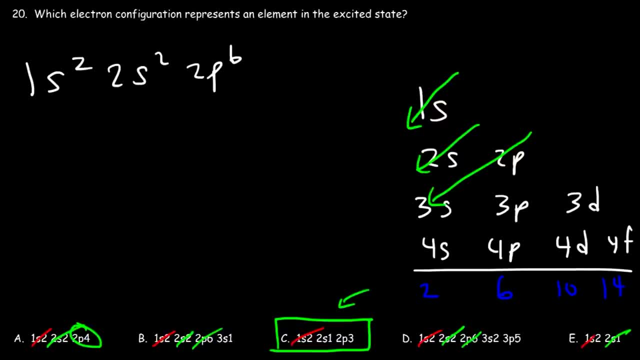 Except this one. So if we were to draw the orbital diagram for answer choice C, Notice how it would look like. So we have 1s2,, 2s1, and then 2p3.. So when a lower energy level is not filled, 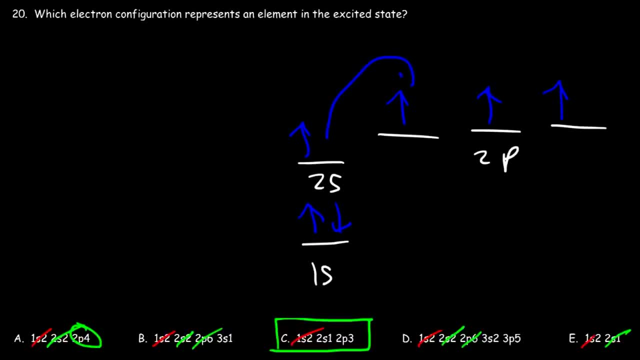 Then that means that this electron jumped to a higher energy level, So it's no longer in the ground state, It's in the excited state, Every other configuration. if you draw it, It's going to be completely filled from the bottom to the top. 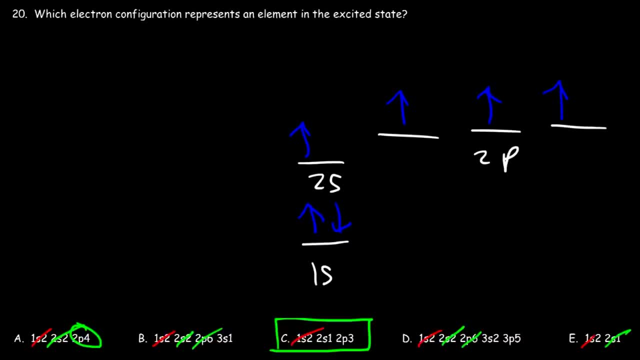 There's not going to be any jumps, So let me use 1s2,, 2s2, 2p4.. So the 2s is filled And there's 2p4. So, as you can see, There's no missing electron in the lower energy levels. 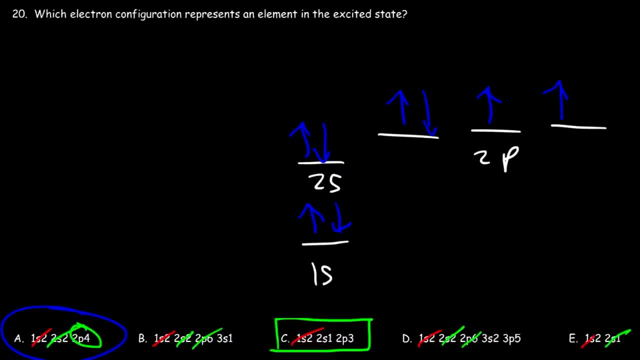 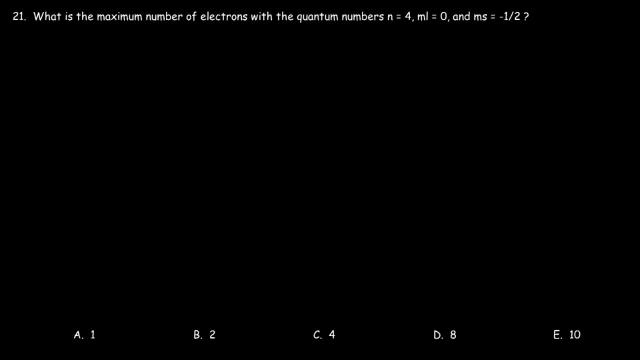 Which means This is a ground state configuration, Whereas this one is in the excited state Because an electron was missing in the lower energy levels 21.. What is the maximum number of electrons with the quantum numbers? n equals 4.. ml equals 0.. 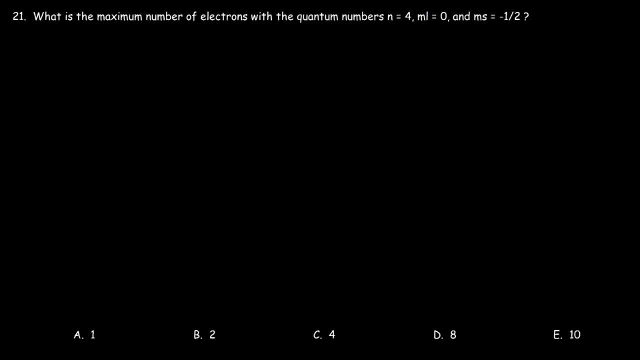 And ms equals negative 1 half. Well, let's find out In a 4th energy level. As we know, there are 4 sub levels: 4s, 4p, 4d and 4f. s has 1 orbital. 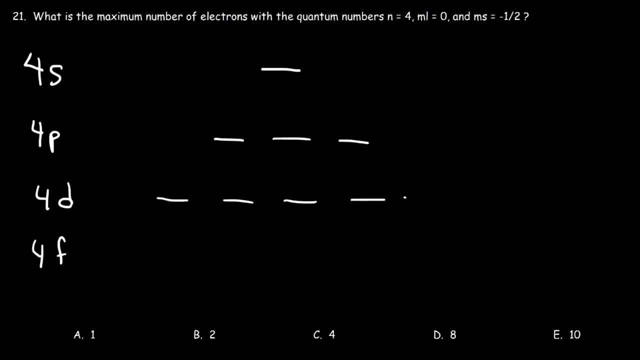 p has 3.. d has 5. And f contains 7.. Now for s, l is 0.. For p, l is 1., For d l is 2. And for f l is 3.. So ml for the s sub level can be 0.. 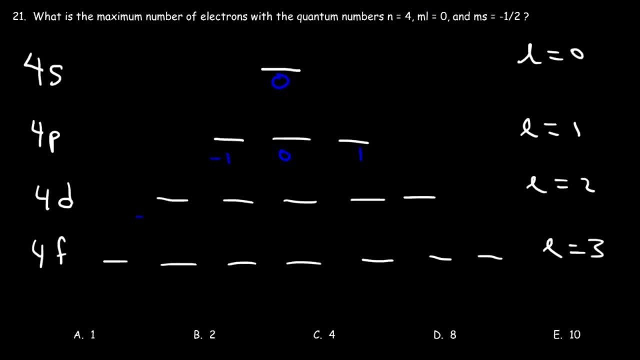 For p, It can vary between negative 1 and 1.. For d, It can vary between negative 2 and 2.. And for f, It can vary between negative 3 and 3.. So now We need to focus on. 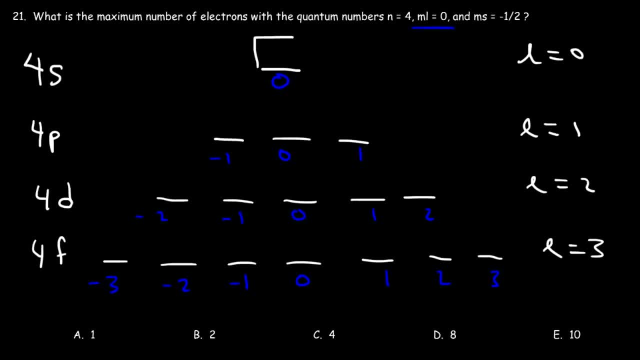 The orbital with an ml value of 0. So those are the ones that are right in the middle. So we have 4. Of these orbitals, And the spin has to be negative 1 half. So we're dealing with An arrow that's facing in the negative. 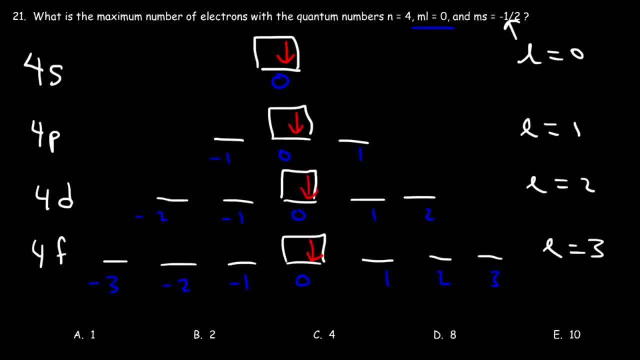 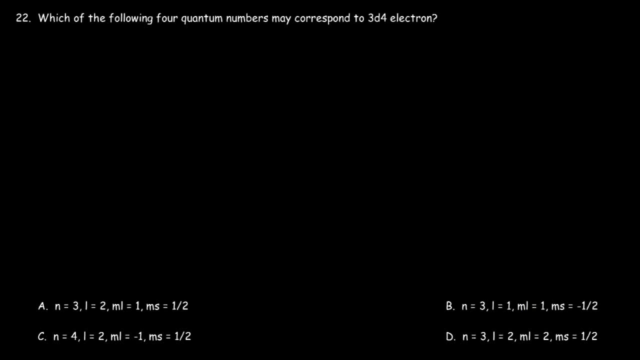 Or in the downward direction. So there's 4 of these electrons That have these 3 quantum numbers, So the right answer is c 22.. Which of the following 4 quantum numbers May correspond to The 3d4 electron? 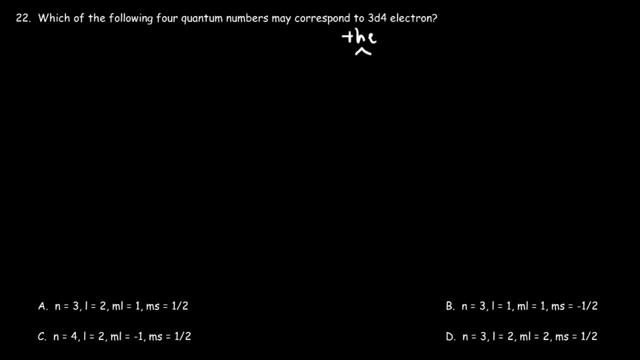 I forgot the word The, But It's supposed to be there. Now, the first thing we need to look at Is the energy level, So we can see the 3 in front of d. So therefore n has to be 3.. 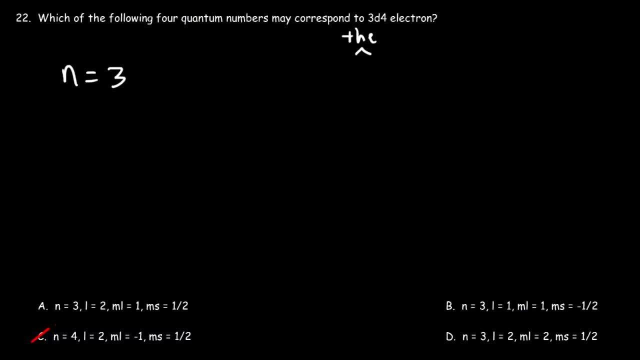 Which means We can eliminate answer choice c Because It has n equals 4.. Now for the s sub level. We know l is 0.. For p, l is 1.. d, l is 2.. So we're dealing with the 3d4 electron.